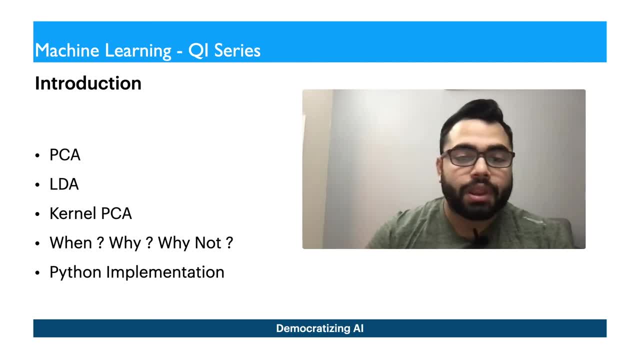 technique over another, and why not use one technique at all? and we'll also see the Pythonic implementation of it. So, ideally, coming to, why do we need this dimensionality reduction, right? so one very common answer is that you know it makes your model very complex actually, and the model tends 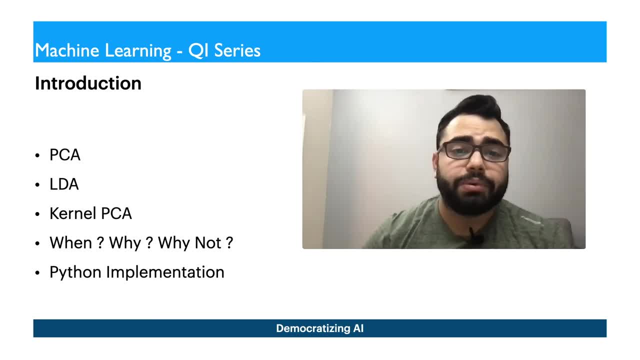 to overfit model is never able to understand on the numerous features, no matter what x model you bring into into. you know action and no model is going to understand the fit, the features really well. So somehow you know to handle the overfitting 19-15- eighth thumbs. we say this that you know. we need dimensionality reduction and this is where you 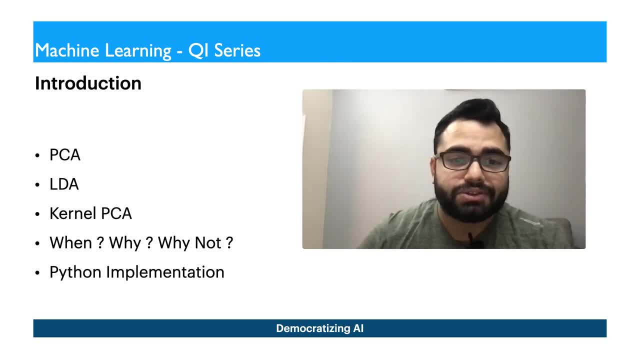 know people say it said, actually it's not. people tell you that actually, that it's a curse of dimensionality as well. So, yes, the curse makes the our model here. Add good wifi access b, tweetedת し c. But ideally, you know, it's very common to have, you know, access of thousands of years, of thousands of features of or 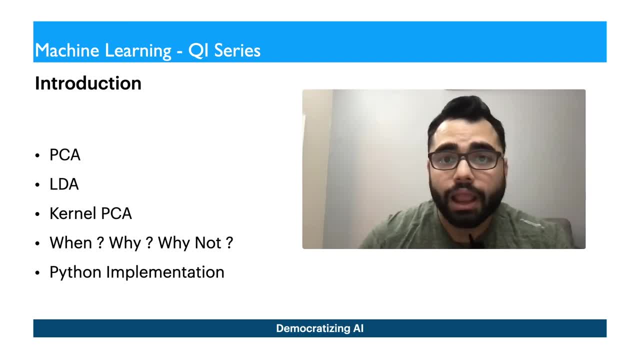 maybe you know one hundred of thousands of features and not all of them are useful, and you know we'll practically never be able to collect enough observations for any use case, and thus we have never enough data for learning algorithms to predict correctly. now, at one point i'm saying: we have thousands of features. 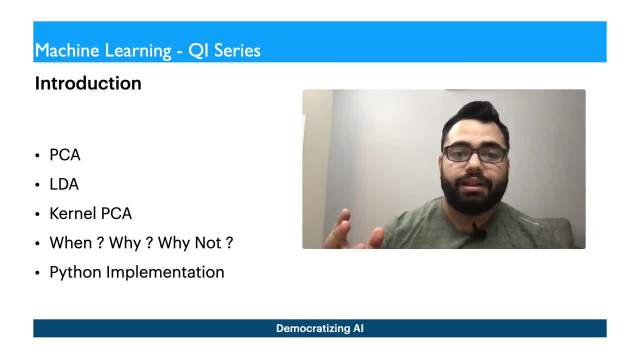 not all of them are useful. at another stage i'm saying we'll, we're never going to have enough data. so what i'm trying to say? right? yeah, that's the curse of dimensionality. you know, it's not always: the more you have it's better. no, it's not always like this. 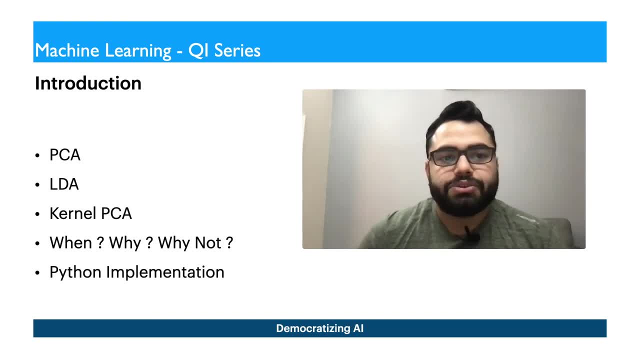 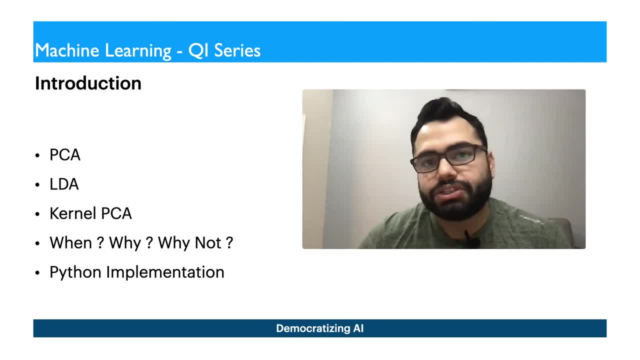 and many more. one is feature selection, feature selection. one example you must have seen in random forest we have feature importance. we can select the important feature there. one is: you know, we can select the features using the statistical techniques like this is the variance, or many statistical tests like ANOVA, chi-square, etc. so ideally, goal of feature. 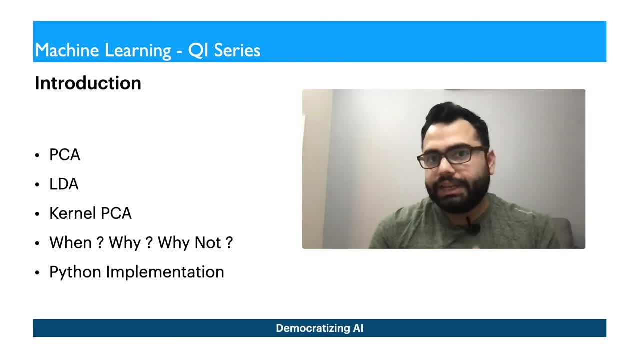 extraction is to reduce them, is to reduce the dimensionality and transform our set of features so that the new features that we have is, you know, it's less than the original features, while still keeping the underlying information intact. and that is what, you know, PCA does as well. putting it another way, we reduce the number. 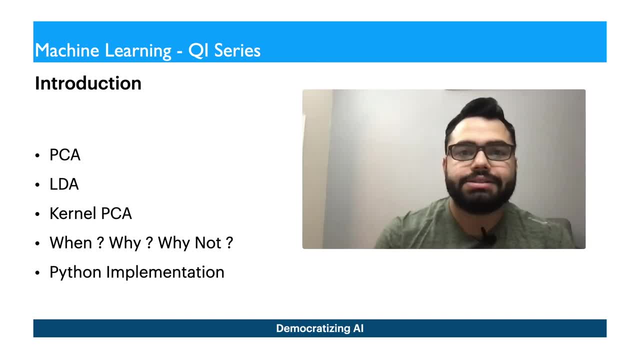 of features, with only a small loss in our data's ability to generate high quality predictions. getting my point? so, whenever we reduce the number of features, we reduce the number of features, with only a small loss in our data's ability to generate high quality predictions. getting my point? 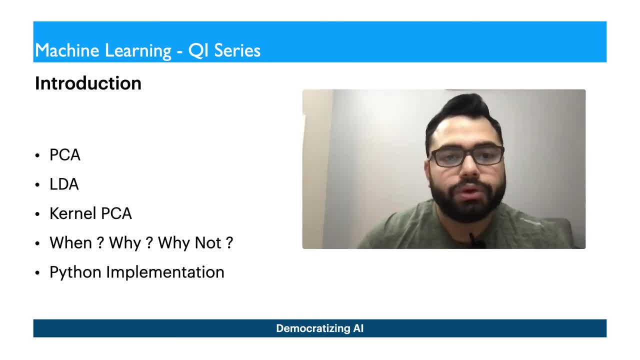 so, whenever we reduce the data, there is still a data loss and but we try to, you know, minimize it. we can say that data- the components, the principal components, or the reduced dimensionality that we have created or projected on another plane- retains around 99.99% of the data. so 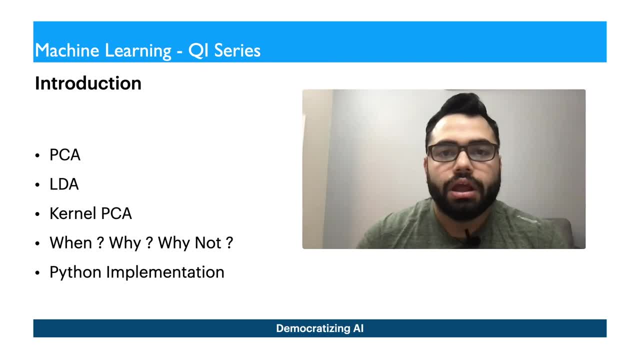 that is what you know we. that is something that we bank upon now. only one drawback is: the new features are not interpretable by humans and will just appear as a series of random numbers. so that's why you know it's complex to explain, as well to maybe your clients. 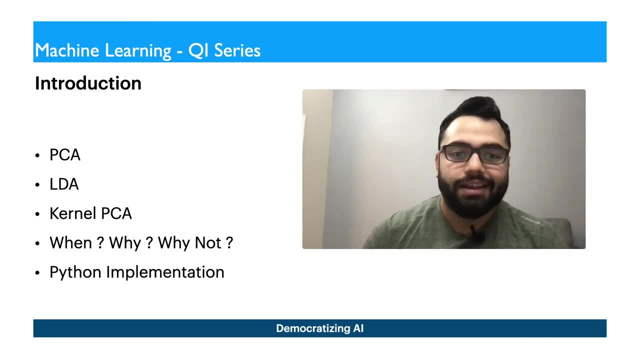 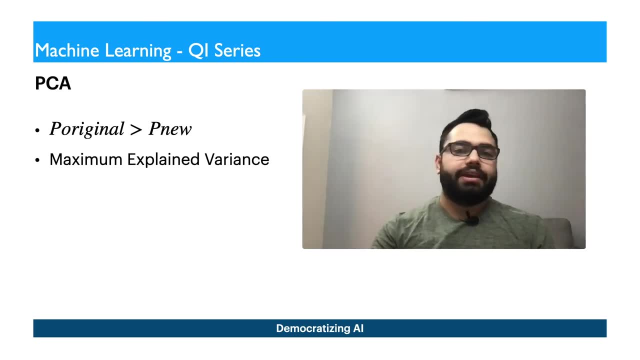 or maybe for yourself to understand it first, and later on you can explain it to your clients if you can. so the first technique that we'll look at is PCA. PCA is again principal component analysis and it's a very popular linear dimensionality reduction technique- see PCA, you know projects. 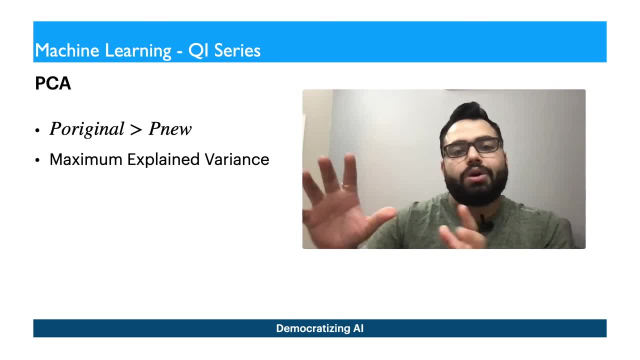 observations you know, onto a principal components of the data, The feature matrix, that retain the most variance. so what are these principal components? we'll just have a look. so now, since it projects the data you know, bases no assumption on a on another principal components or a vector. you can say that's why it's a unsupervised. 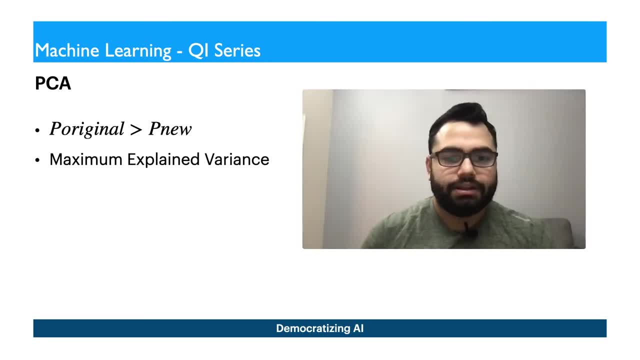 technique, unlike LDA, which is a supervised technique, we'll just see in the tutorial. thus, PCA is a unsupervised technique, Meaning It does not use the information from the target vector and instead only considers the feature matrix. so that's a very important point to remember. now for a mathematical description. 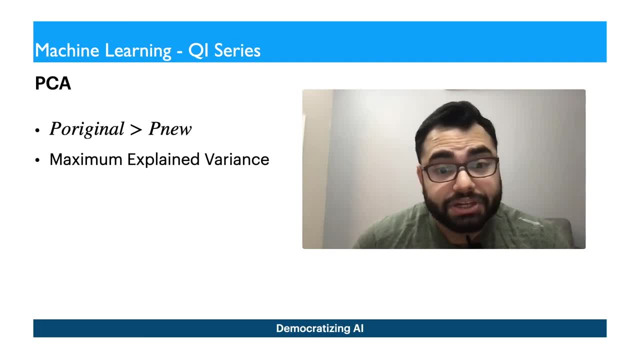 of you know how PCA works. I'll just mention some external resources and maybe I'll try to explain some bit of mathematics as well, if I'm able to. and then you know, maybe basis that mathematics you will get some intuition behind PCA using a simple example. 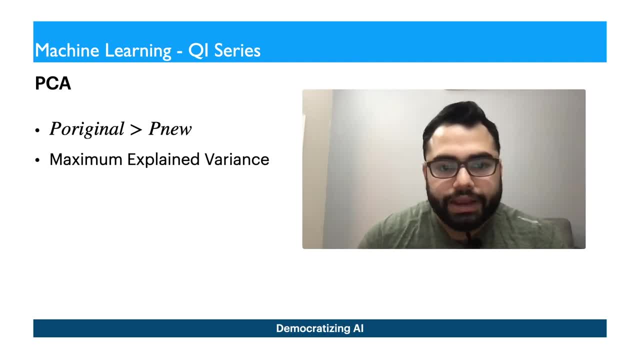 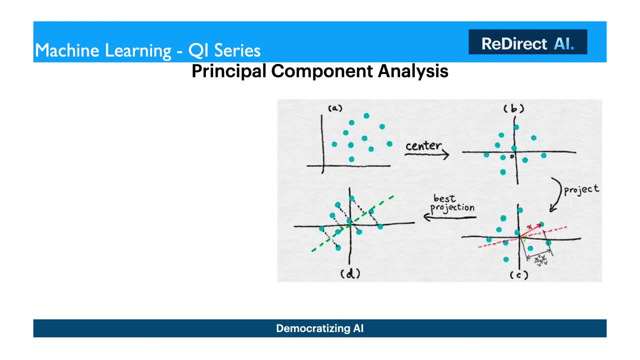 So now, in in the coming screen, we'll have a figure. in the figure we'll have, we're going to have two axis, and just let's have a look at the visualization now. so now, so see this first figure a. we have some data points on. let's say, we have two features, only x-axis. 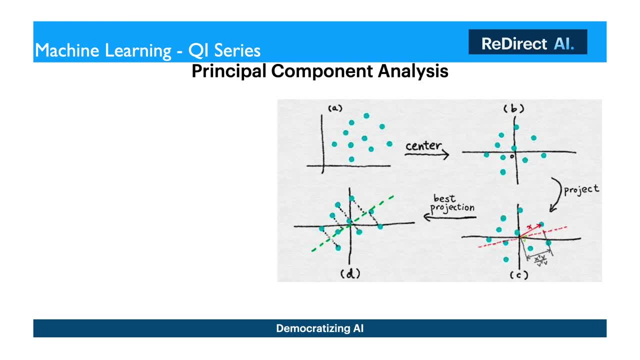 and y-axis and on the figure b you see the axes have been changed so and it says center. so you know PCA centralizes the data first, it will bring the data to the center and it's it takes this assumption that data has a center. so that's another crucial point about PCA. 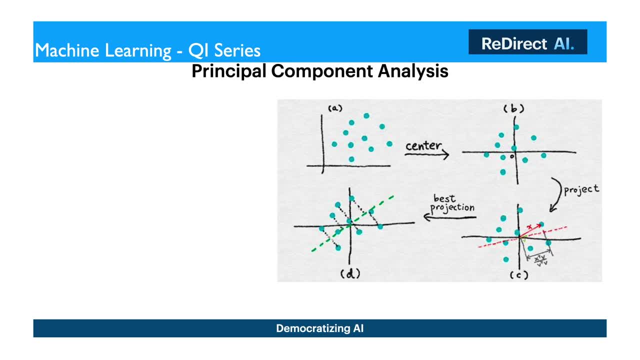 that it assumes that data has a center as well. now, third thing: what it'll do is, you know, it will just do like a regression. as you can see, we have a red line and a red x, so basically it will try to fit a best fit line. as you must have seen in regression ordinary. 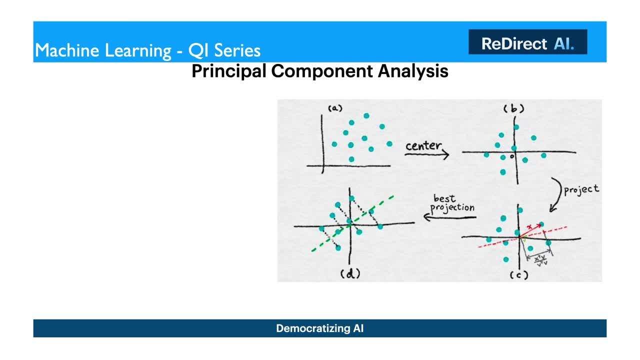 least squares. that is what you know PCA also does. it creates a best fit line and tries to project those points. So now we have a new vector or a new line, whom we call principal component, as you can see in the figure d that the green line has the projections. and now these projections: 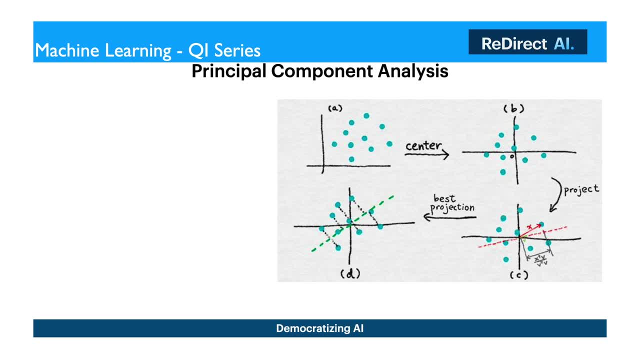 where these points, these dotted lines, are cutting, the green line becomes the representation of the actual data. so it takes two major assumptions: that it centers the data and it fit, and it fits a line. now, finally, what's its? you know, the last functional, you can say the cost function. 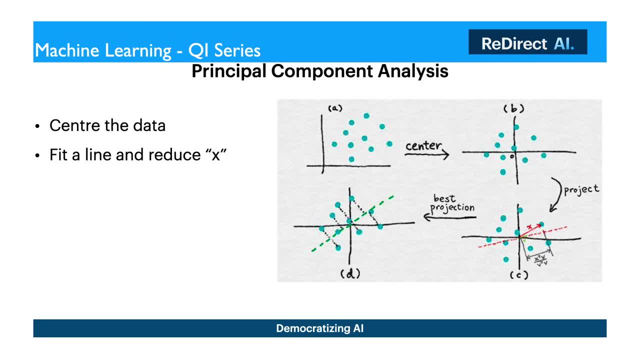 maybe I've already explained in a separate tutorial what a loss function or what a cost function is. so ideally, here our cost function is x. it tries to reduce the x. now why x? you know we already have a projection to this from our point to the green line. we already 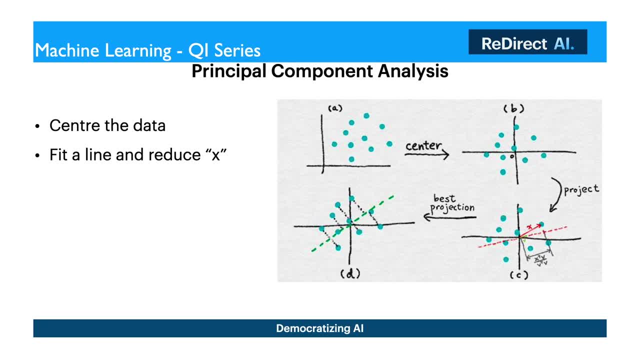 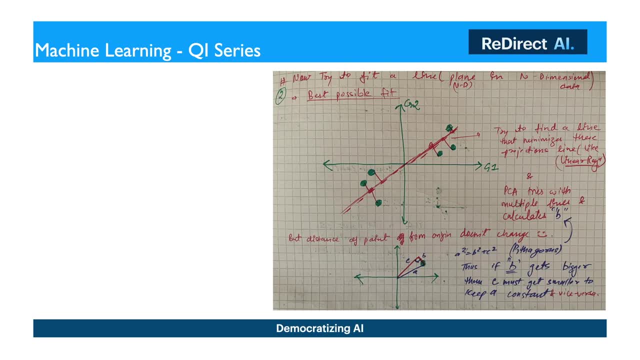 have a projection, but why does it want to reduce x? so yeah, I have prepared some notes for it. so let's assume you know you have this data, whereas you have two features: g1 and g2.. As you can see, the green dots are the actual points, the red one is the principal component. 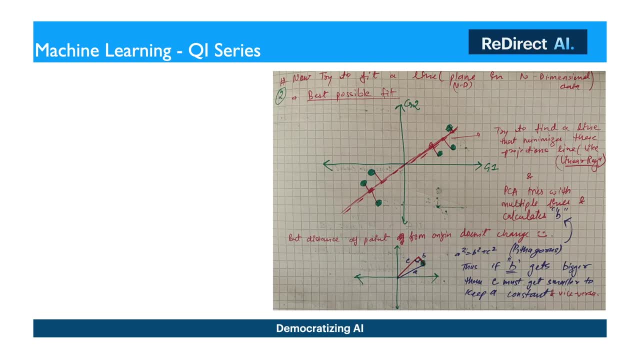 and we'll try to find the line that minimize these projections. all right, but as I said that we'll try to minimize the x, now we'll just see where this x is in the figure below. you see that. you know I have created a triangle like a, b and c, where a happens to be the hypotenuse. 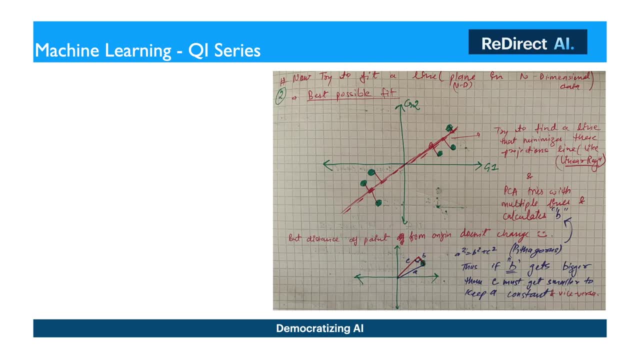 and b and c happens to be the other sides of the triangle. so ideally we have this relationship of: a square is equal to b square plus c square. now this a is fixed. okay, whether we centralize the data or we do anything, that the relationship between other points going is going to remain. 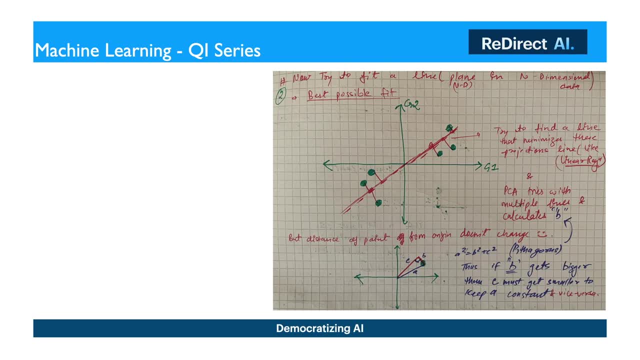 the same. so that's why the distance from origin is going to remain the same. actually, the relative distance from origin is going to remain the same. thus we are left with b and c. now if I say that you know, if b gets bigger, then I think we don't have a best fit line, because 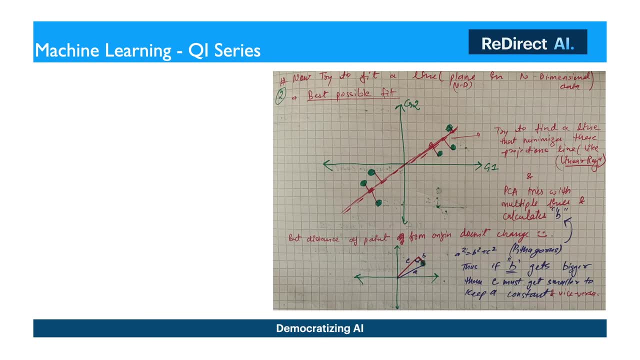 the projections are very far actually and our cost function is to reduce b. all right, we try to find the line that reduces b. if we say that we want to reduce b, then I would say: you know that we try to find the line that maximizes c or vice versa. that I've written. 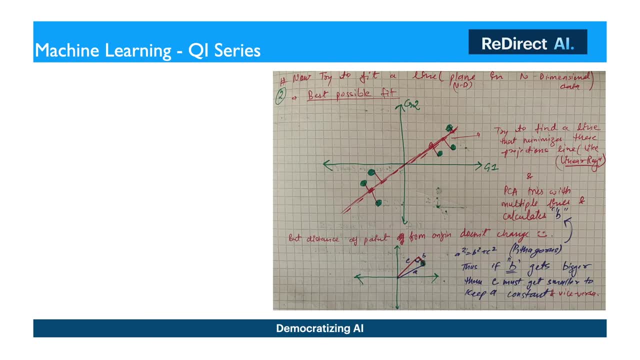 is: if b gets bigger, then c must get smaller to keep a constant, vice versa. so vice versa case that we look upon is reduce b and maximize c. And why c? because competition of c is cheaper. that's why you maximize c and thus, and b gets. 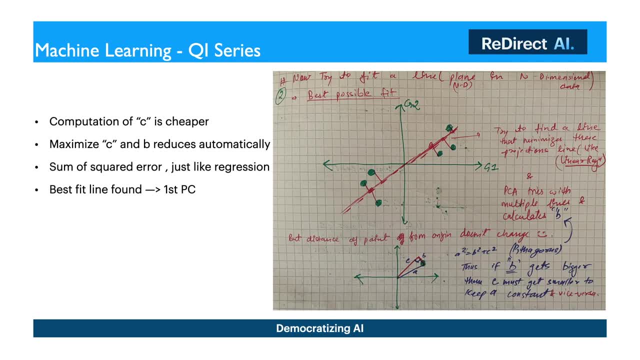 reduced automatically. now, what is this? b is just simply, we put it as sum of squared error, just like rotation square, because you know it tends to get positive values and we are interested in distance metric, and then not its magnitude, not its orientation or polarity. you can say: 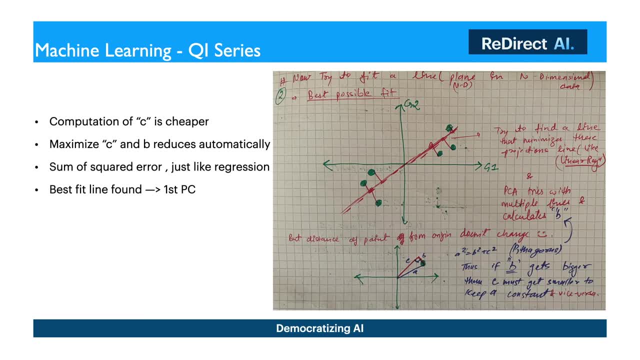 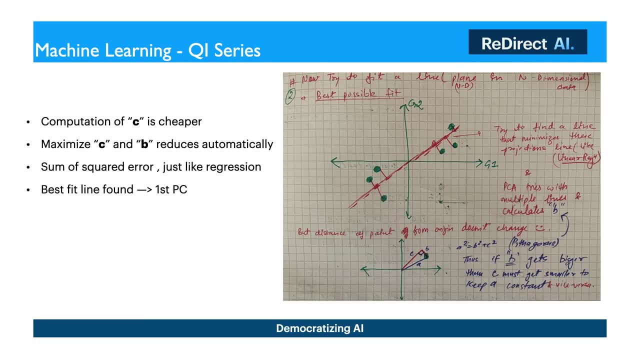 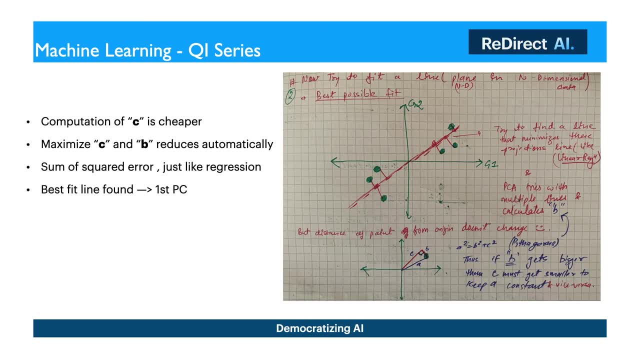 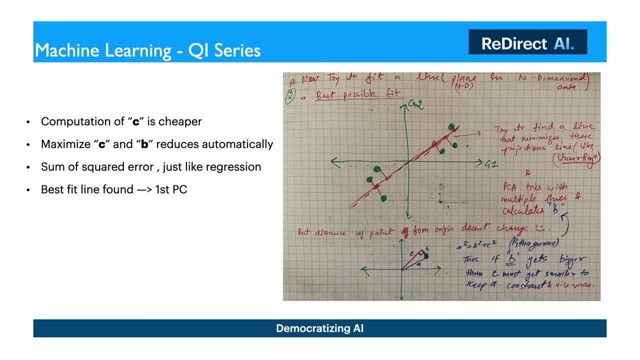 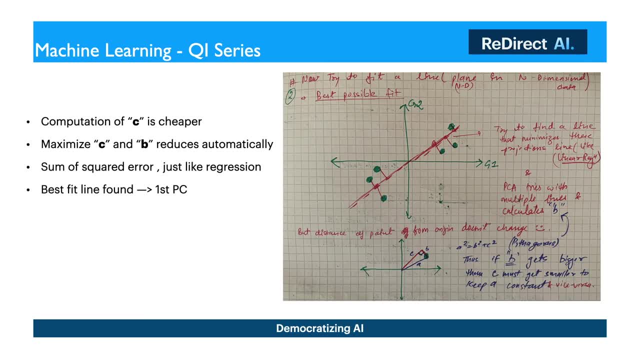 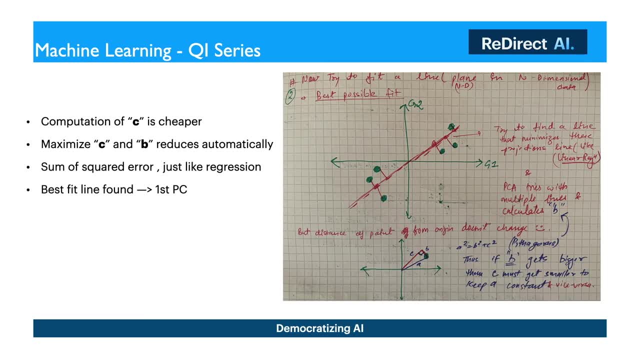 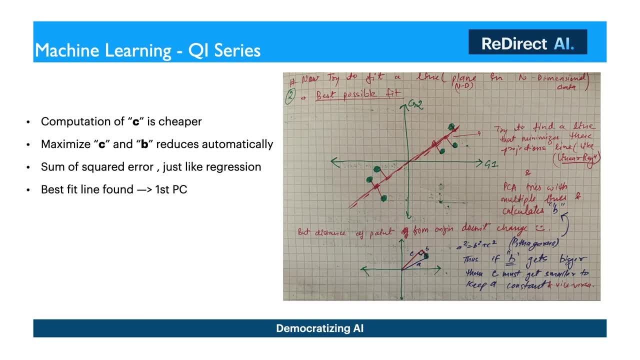 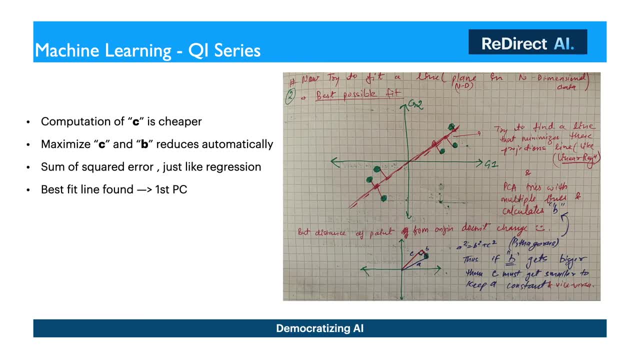 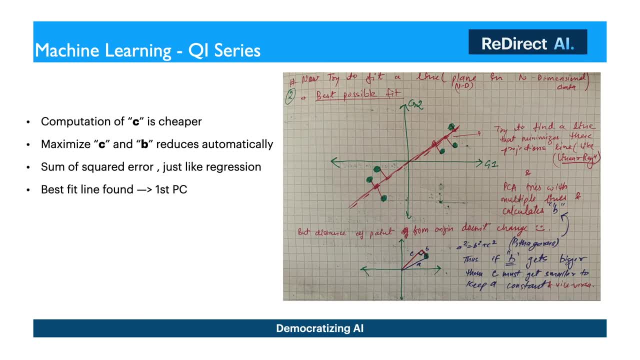 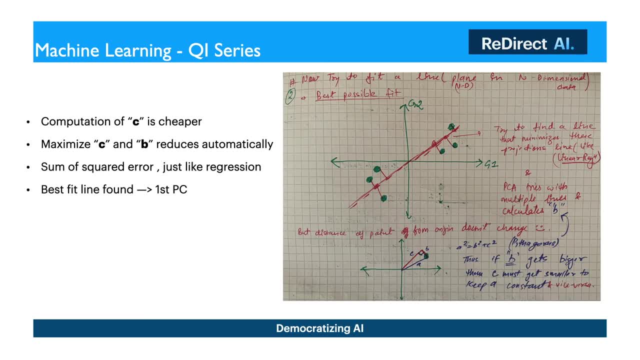 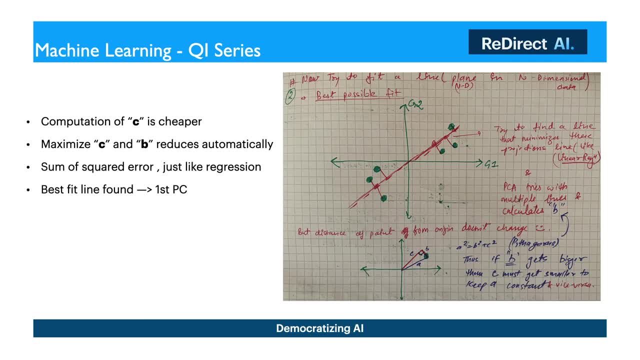 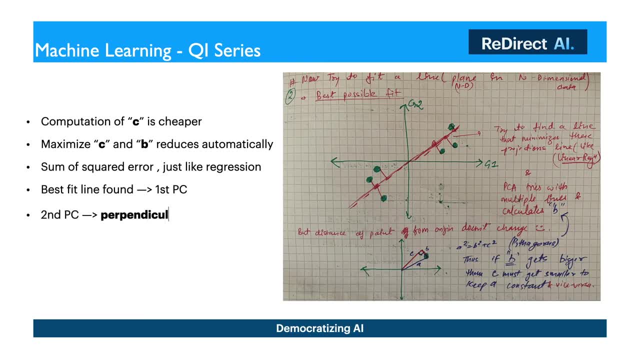 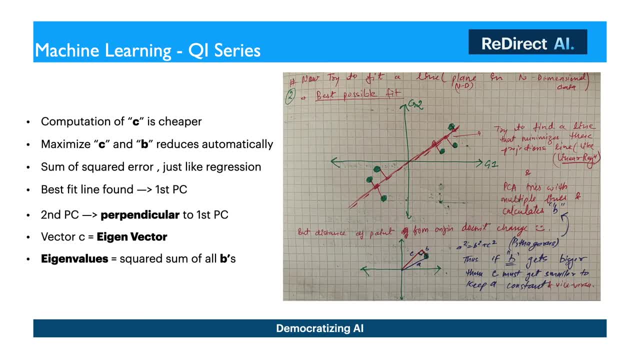 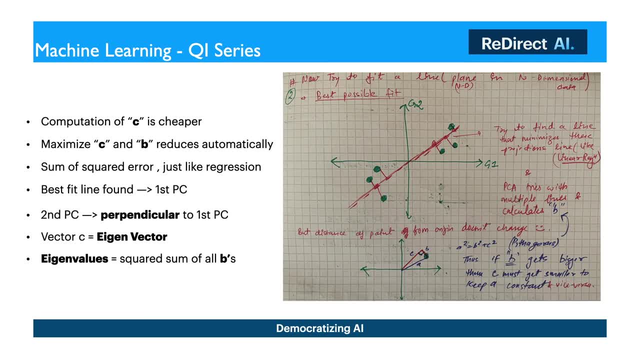 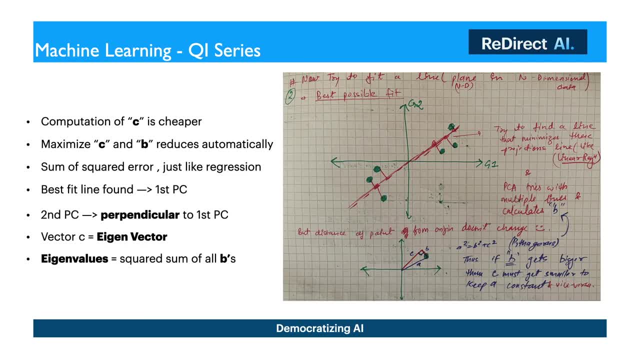 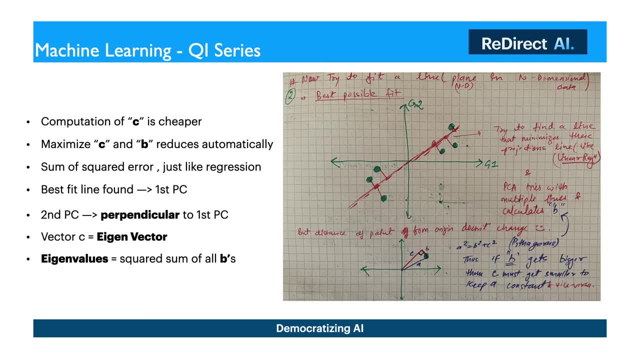 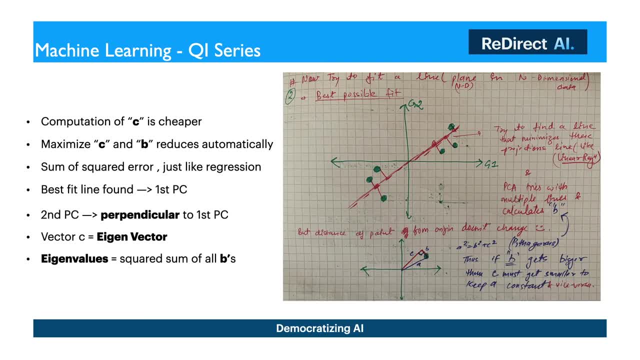 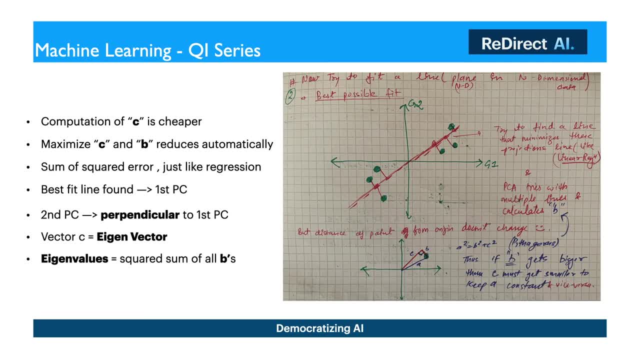 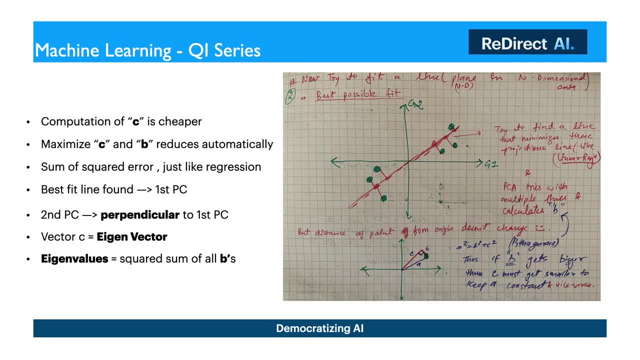 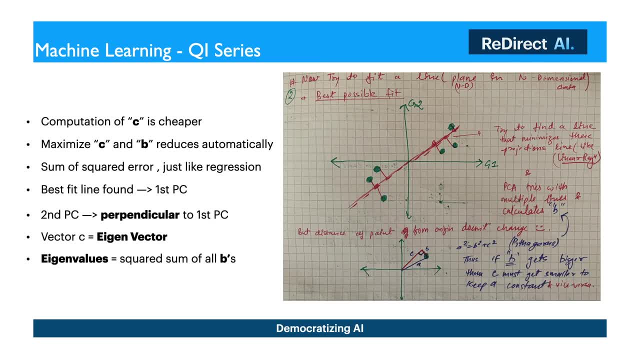 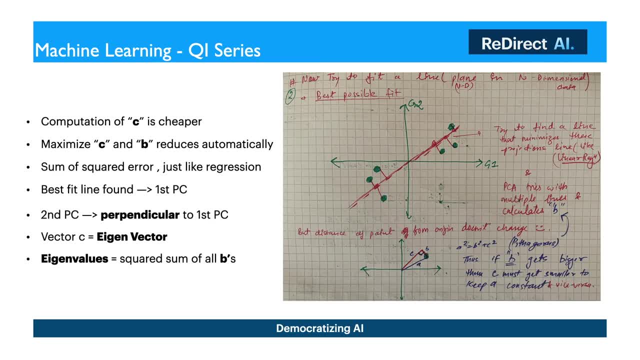 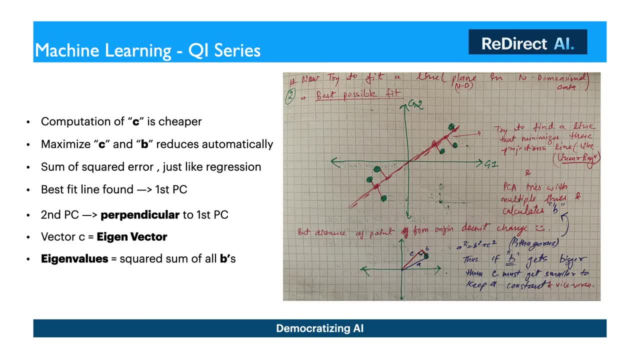 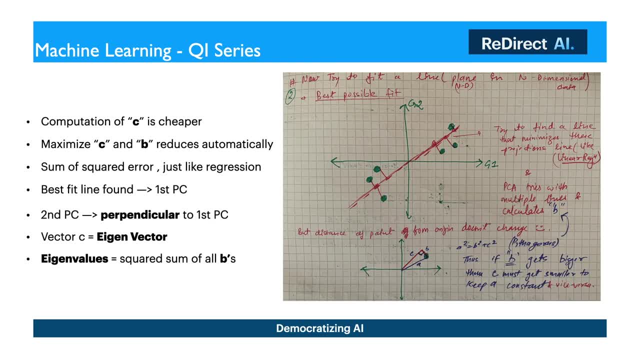 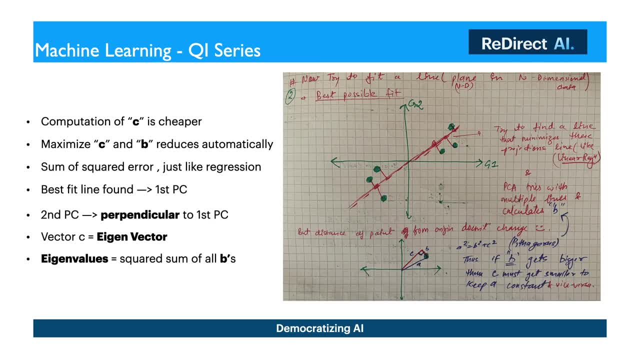 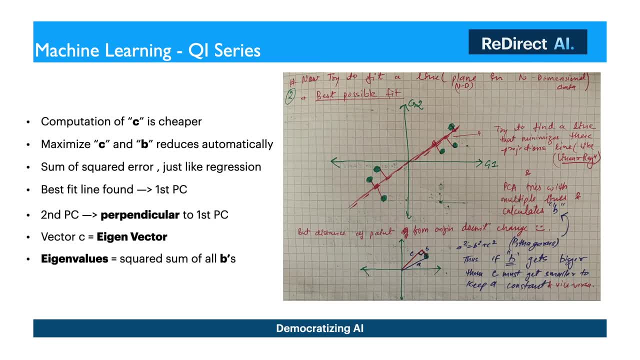 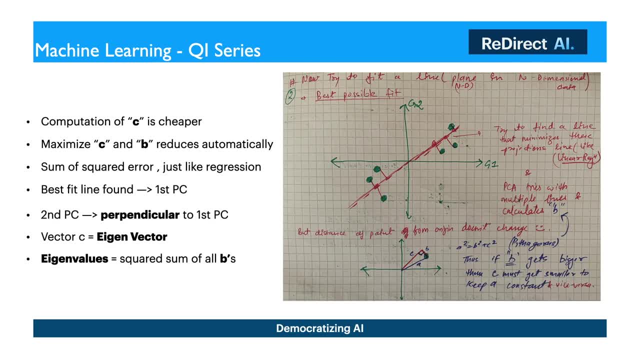 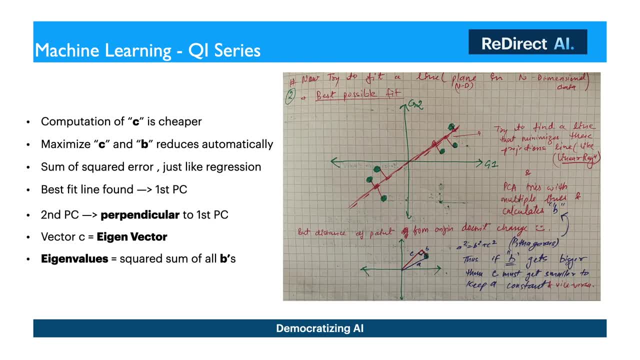 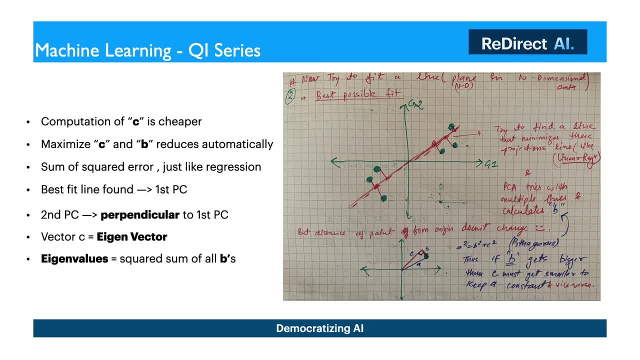 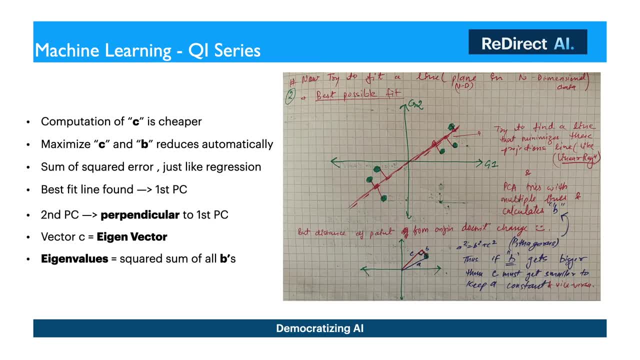 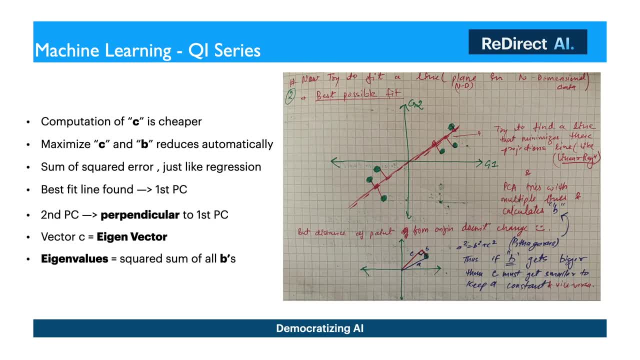 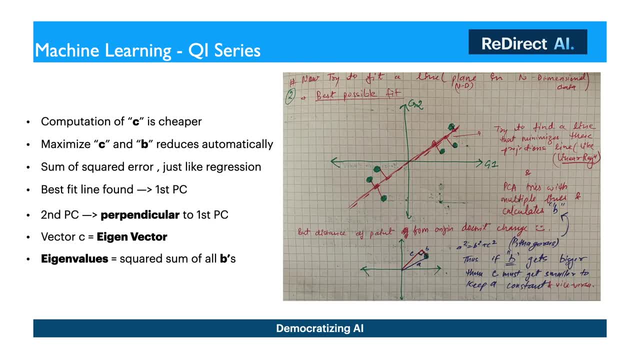 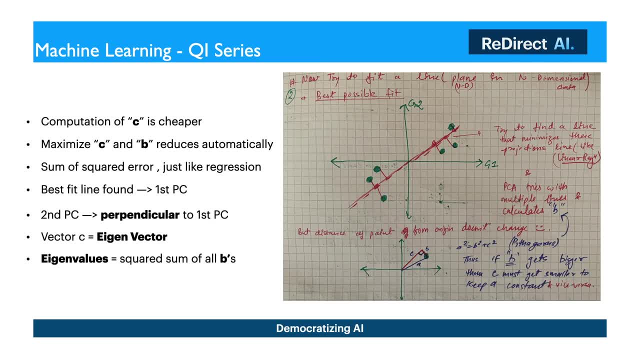 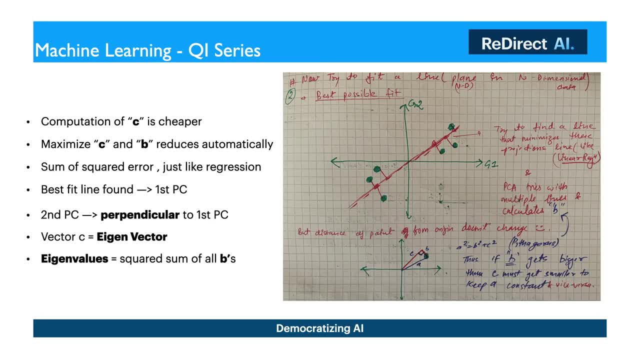 And the best fit and line found would be our first line. And the best fit and line found would be our first line parameter called Witten, you know, which transforms the value of each principal component so that they are zero, mean and unit variance. this is, these are some. 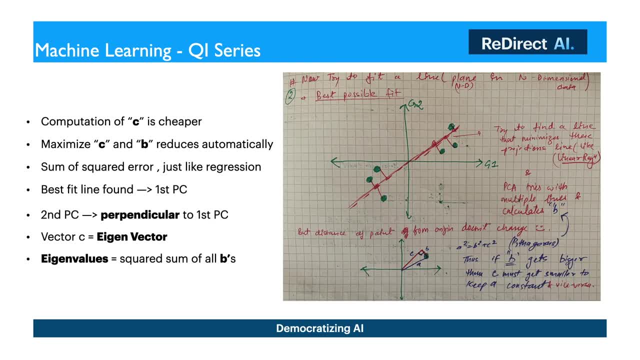 statistical terms. but not need not, you know, worry about it, it's fine. another parameter and argument is SVD solver, which ideally we keep it, you know, we try to keep it as randomized. SVD solver- randomized, you know, implements a stochastic algorithm to find the first principal components and often 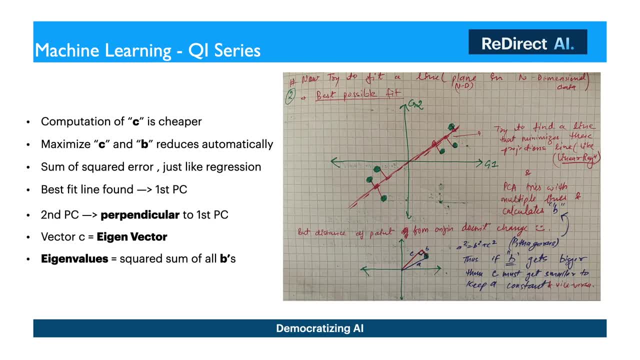 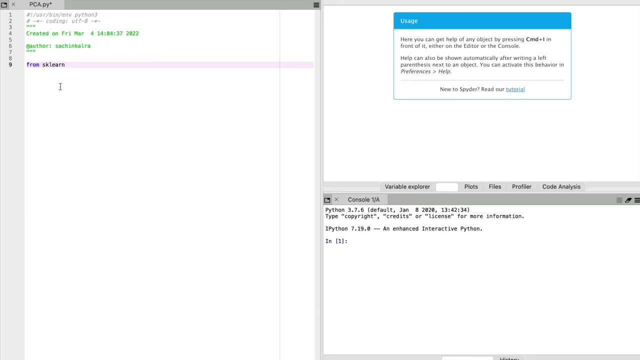 significantly, significantly less time, since we are computing C, which is, you know, the cost of computation is very less, but it still takes a toll, you know, if you have a large dimensional data space, so yeah, let's implement it and see how it goes. all right. so I'll just, you know, load the standard scalar first from: 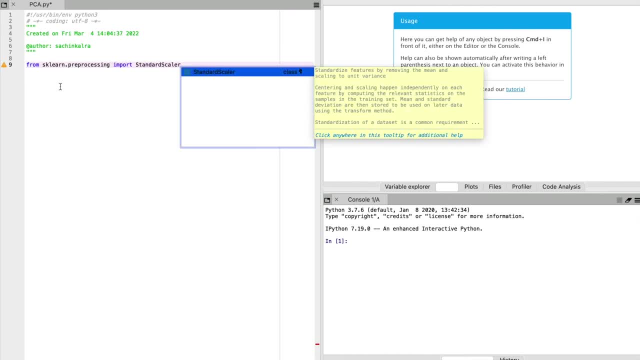 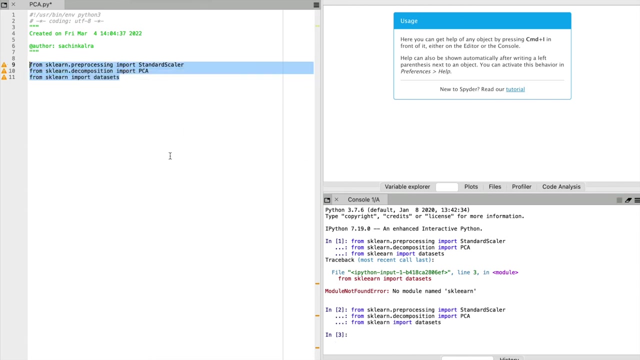 pre-processing for the Z transformation, because we want feature on the same scale. and now I'll just call the PCA from the decomposition, which holds the functionality for PCA, and finally I'll call the data set as well. now let me just run it and no module. oh sorry, I made a mistake. yeah, let me just run it again, all right. 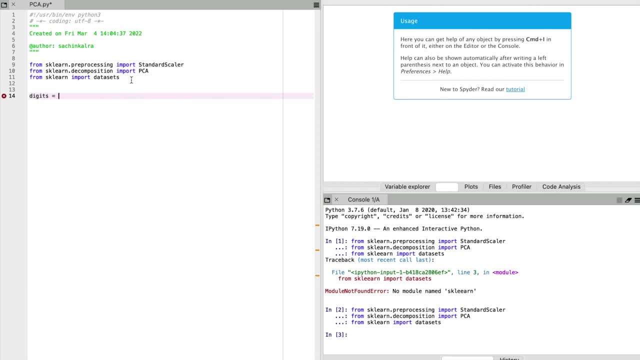 then now we're using the digits data set today because it has very high function dimensionality. just you can load it and we'll use the feature return X, Y. true, you know, it will unpack into features and target. yep, that's right. so you have features. you see these? we have 64 columns and 1797 rows. 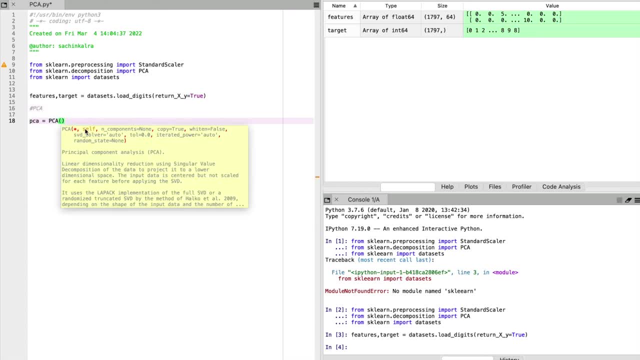 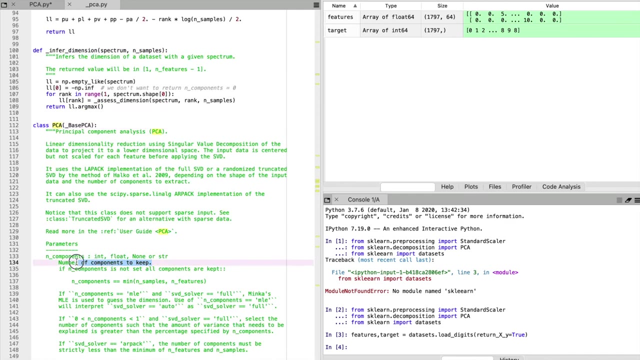 I just apply the PCA and I'll initialize it. you see, we have the same components or parameters that we discussed. we can also, you know, access the documentation. let me, let me show you just a second. so if you don't have any documentation Documentation handy from scikit-learn, you know, you can go to the internal downloaded documentation and like a multi-line comment. 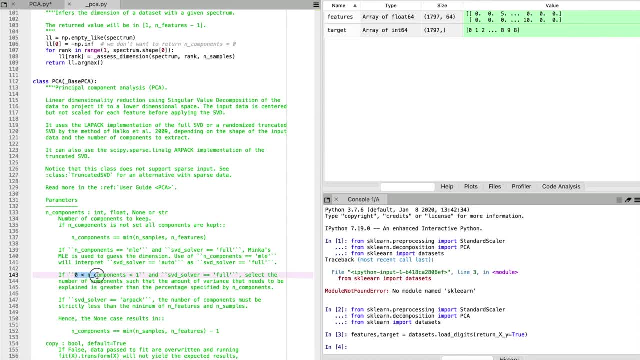 So we have like number of components That's between 0 to 1.. It will be, you know, the variance, the amount of variance that needs to be, you know, explained. If it's more than one, that will be number of components. We'll try both. 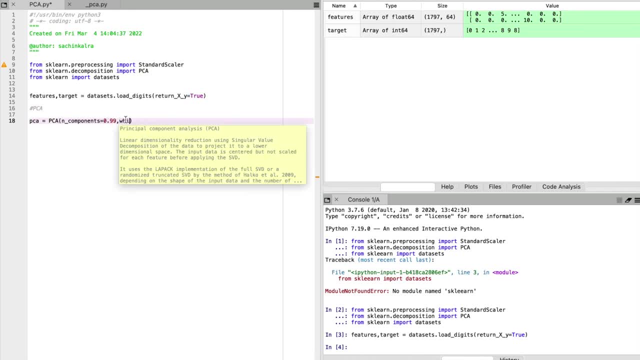 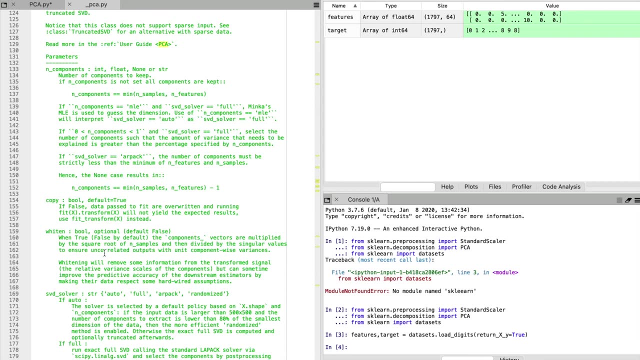 I'll just keep it at 99. It means 99% within equal to true. So it's another happy parameter. We'll just again have a look again. So it's basically you know Scales, the components, so that we have, you know unit component twice variance. 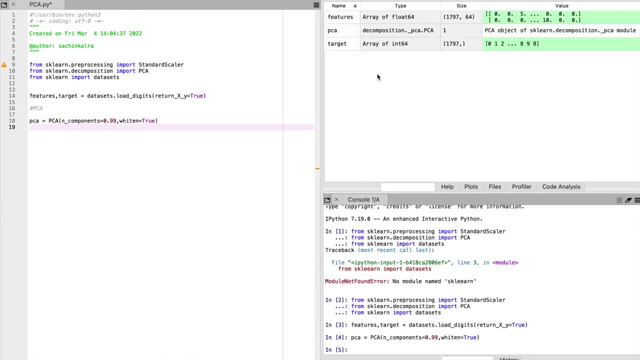 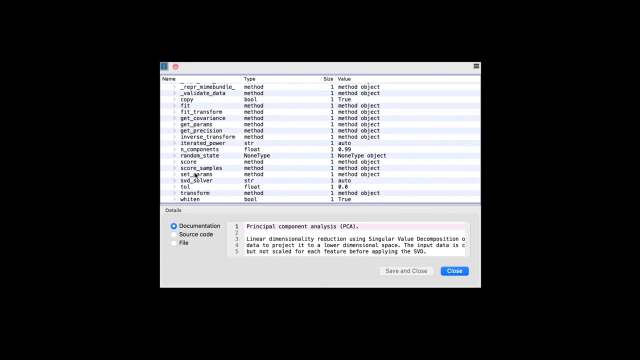 Like unit variance. I would say, Alright, let me run it. So PC has ran and we've got one component and it has multiple features, just like this. I'm just checking in or taking a walk around so you can just replicate the same to get get an idea of how it works. 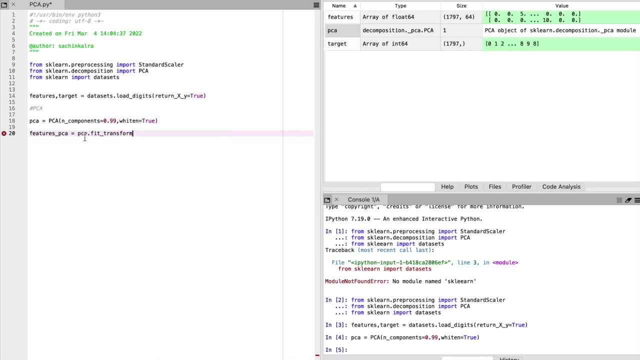 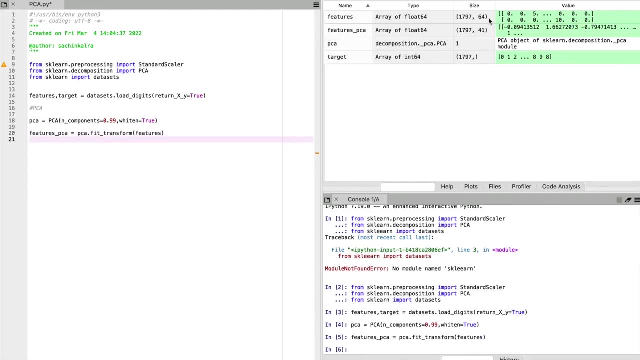 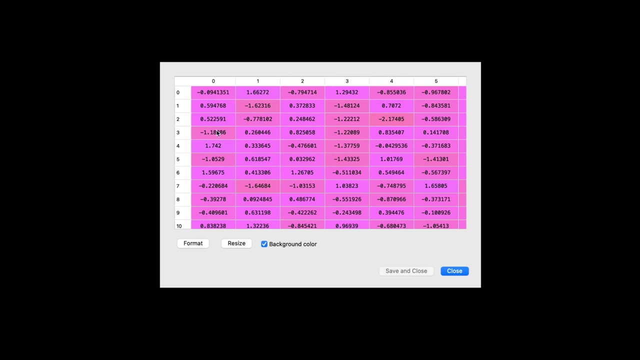 So we'll just transform the features, Or fit, transform, and we just pass on the only features, no target, because it's a unsupervised technique. So we've got 41 features now reduced by 23, and so earlier it was like this, now It's like random numbers. as I said, positive, negative, real numbers. 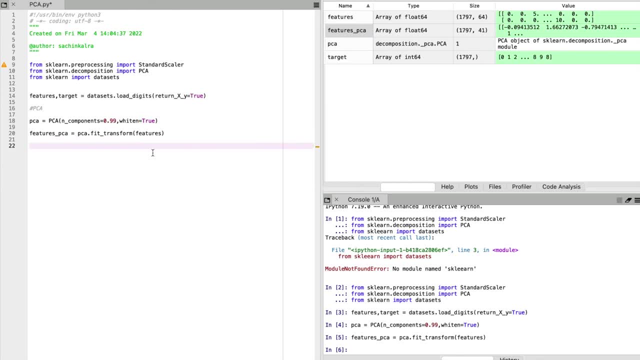 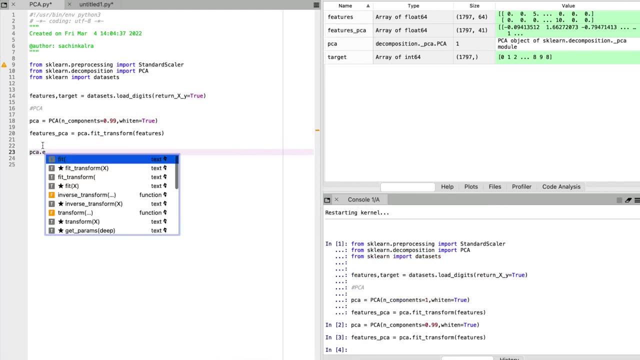 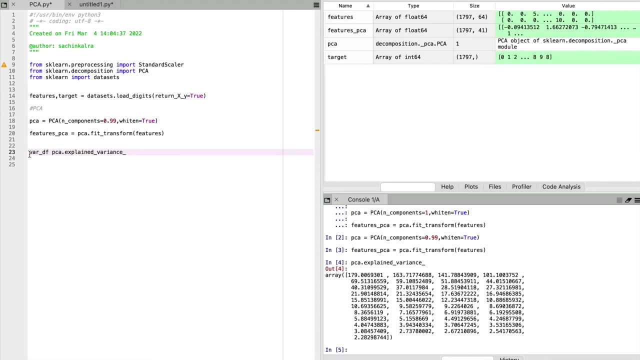 Are very difficult to explain. but yeah, it works. Now We'll just have a look at the explain variance. now Access is accessible by the attribute explained variance. So, yeah, it gives the explain variance of all the- you know- 41 components. I'm getting call it, you know, you know, in a separate data frame. if you want, you can check the dimensions as well. 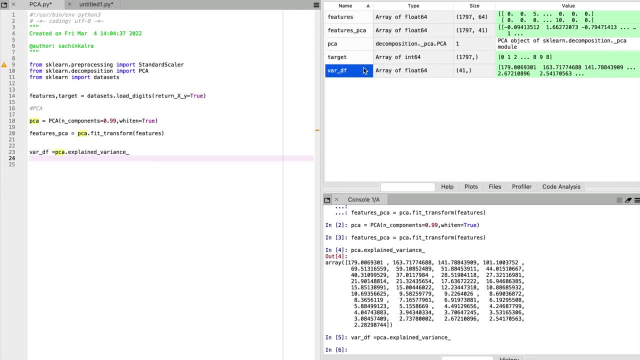 So, yeah, it has got 41 dimensions. now, Again, these are random numbers and the magnitude of variance is there. So, how to understand how much of variance is being explained by individual components? We can just, you know, use the explain variance ratio parameter. for that, 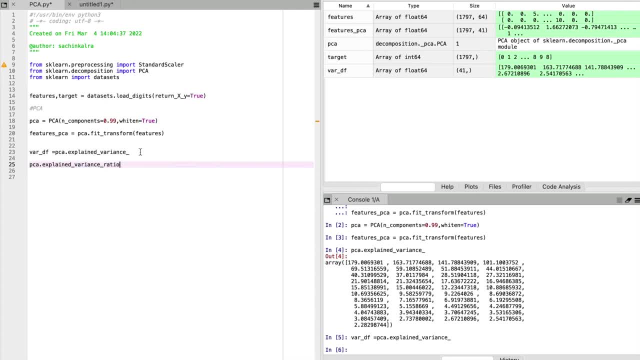 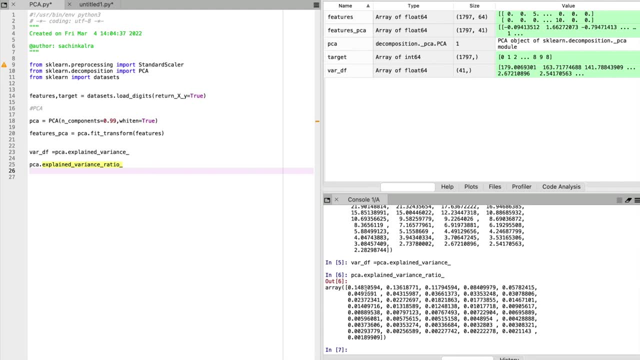 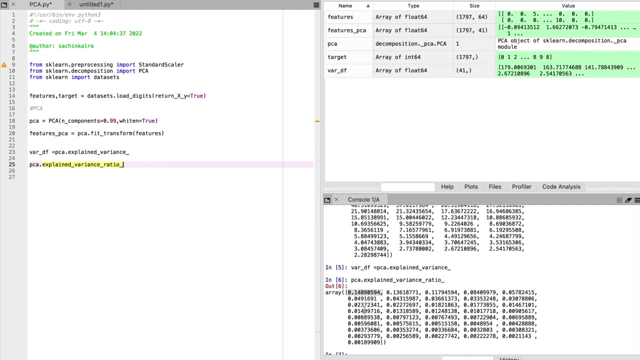 Which you can access by PC, explain variance. our ratio underscore And we'll just run it. Yeah, we got it. So if you'll just sum it up, you know it will come out about 0.99. so this is like 0.14 means 15% and 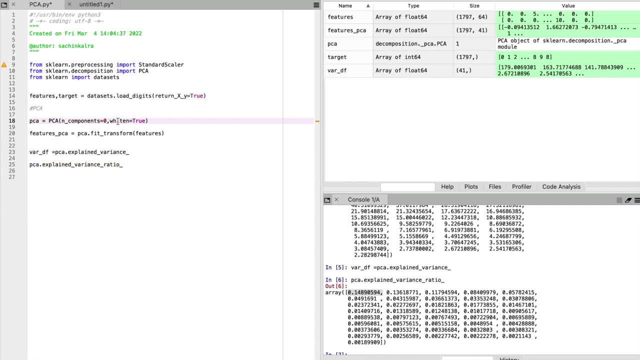 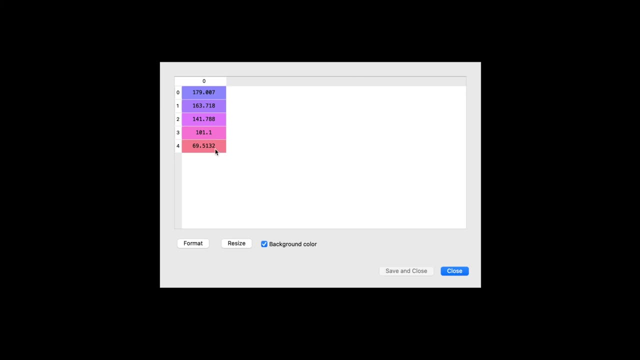 So on, so forth. Now let's try one more thing. Let's, you know, limit the number of components to a 5 and let's see how much- you know- Variance do we get. is it able to capture in five components? We've got five dimensions. yeah, these are the five companies. 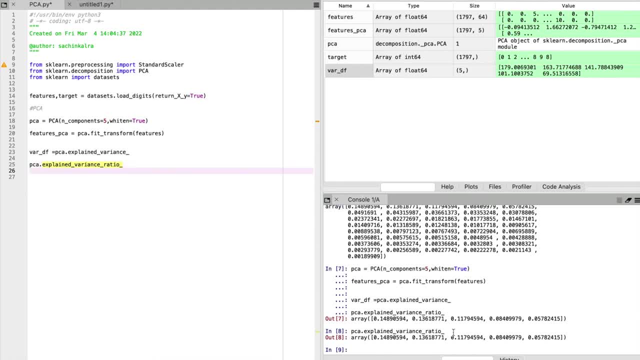 Ratio is already there, Yeah right, So no, we're not able to capture maximum. you know variance in five components, So machine decided that at least we should have 41 components for it. so we'll see in a separate video. You know how do we decide on. how many components do we need so we can make our code, you know. 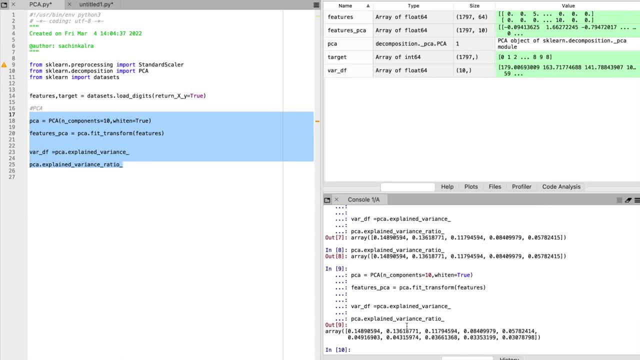 That once we have read certain threshold of variance, stop. and the number of components. So yeah, wit n as well. It hasn't increased much, so No worries, will see in a separate video. I just wanted to show you how PCA works. Let's move on to another technique now. 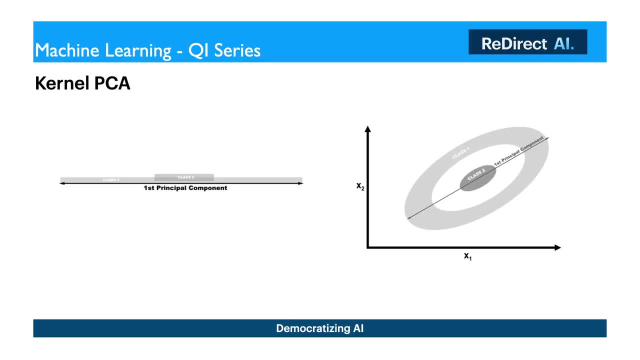 PC is able to reduce the dimensionality of our feature matrix, That is, the number of features, and standard PC uses linear projection to reduce variance, reduce the features we just saw. but what if data is linearly inseparable? what do you do about it? see, when data is linearly separable, we just draw a straight line or a hyperplane between different. 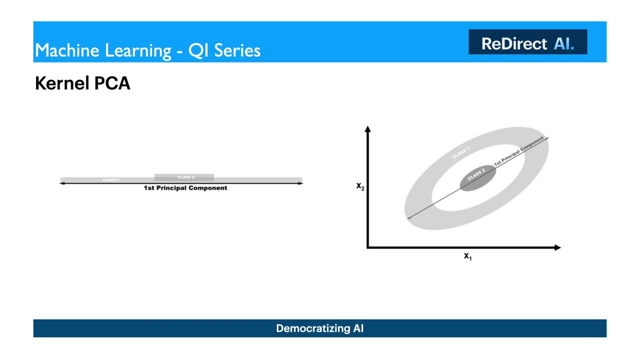 classes and pc works well, but what if our data is not linearly separable? you know i mean? example is that you can only separate classes using a curve decision boundary. so that is what i meant from linearly inseparable data. thus the linear transformation will not work. and what do we do? 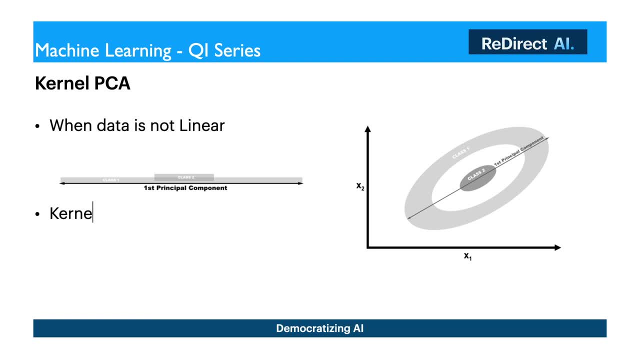 about it. so in this case, you know we'll go with kernel pca. so kernel pca, you know, when data is not linear, it's fine, we can go with the kernel pca, as you can see in the figure that when data is not linear, principal component will mix two classes. and when we have kernel pca, can it can. 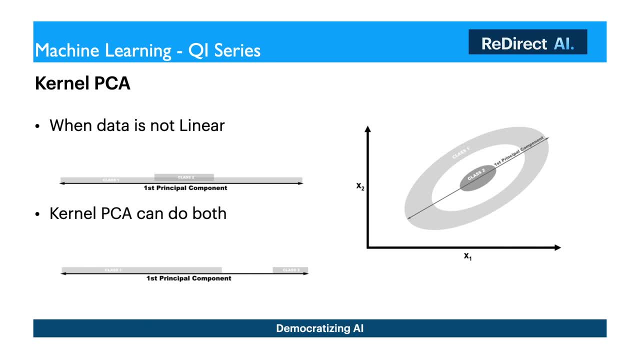 you know, separate the classes. because it can separate the classes, because it can separate the classes, because it can separate the classes, use a feature called it has the functionality to implement the- uh, you know- spherical boundaries. so that's how you know it is able to, uh, separate both the classes and it's a you know better. 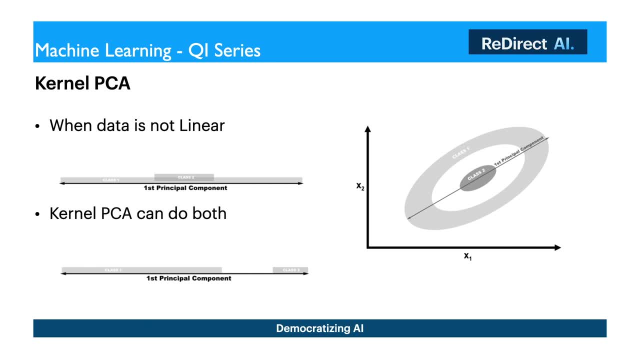 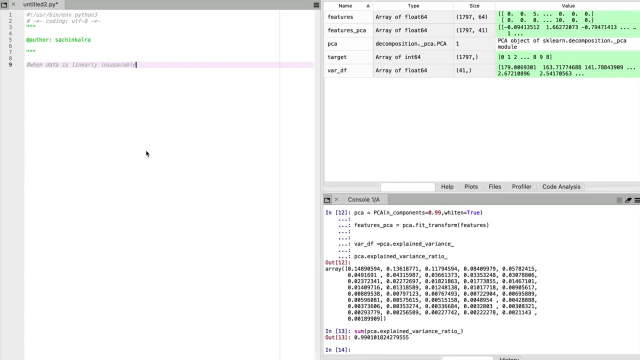 technique over pca. if you have linearly inseparable data, so yeah, let's implement it and discuss further there. so now our data is not linearly, uh, separable. so in our solution, uh, we'll use- you know science, scikit-learn's make circles- dataset to generate a simulated data set. 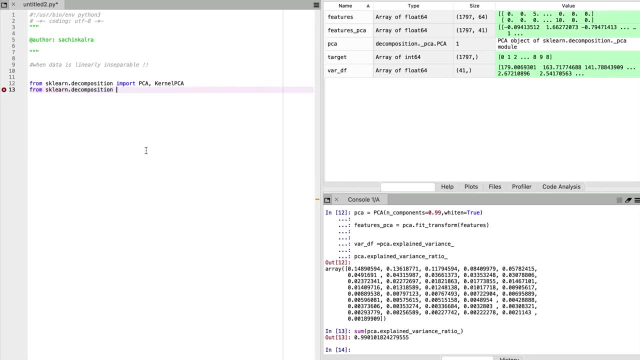 and i'll call pc and kernelPC from decomposition. yeah, so make circle makes the data linearly inseparable. all right, just a second. yep, all right, that's fine, i've got the- uh, my queries in place. i'll just call the features out. now i'm going to ônâş這 절대不 movimento. my process is in place. i'll just call the features out of my learning process to generate Sam술ainí y subjective二重� Corporation baking data and to generate a simulated dataset. and I'll call PC and kernelPC from decomposition. yeah, so make circles makes the data linearly inseparable. all right, it's fine. who got the macrame s worry about you? i'll just call the features up here as my favorite supersלא només cel코n. 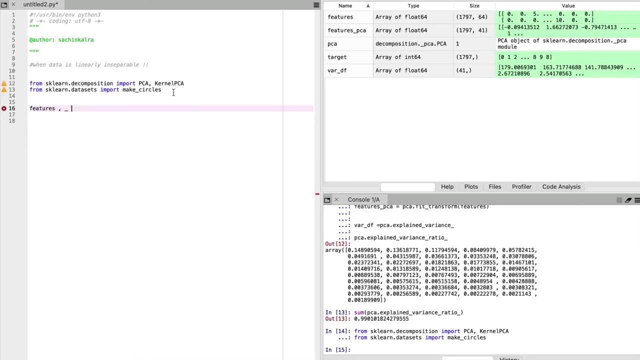 of fields. i'll just call the features and then i'll call it functions and LabsBeta, NBC, and from it we'll get less performance, or So thousands of cloak c quit Delhi university in place. I'll just call the features and you know so it. this is for the underscore, is for the 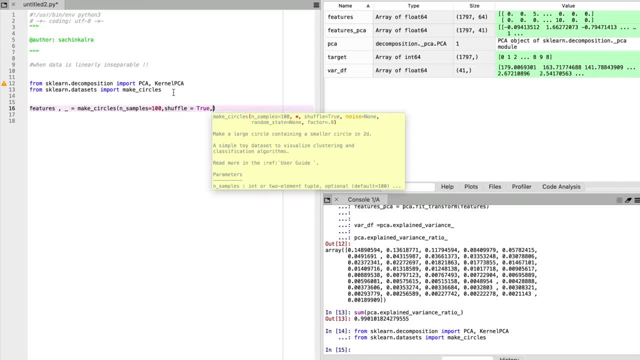 another values that get unpacked. I'll just call how many samples we need. the random state: how much noise do we? you know if you want to introduce or not, and I'll add the factor as well as 0.1. you can read more about it if you want through the internal documentation, just like this. 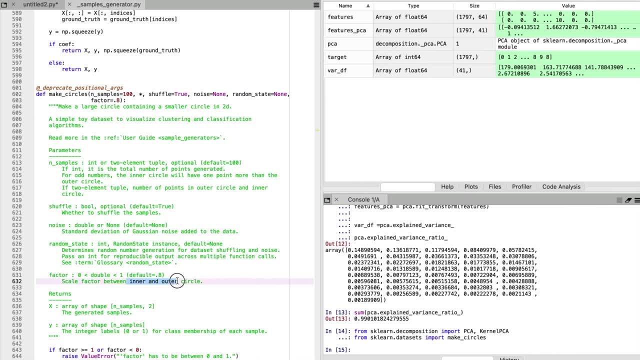 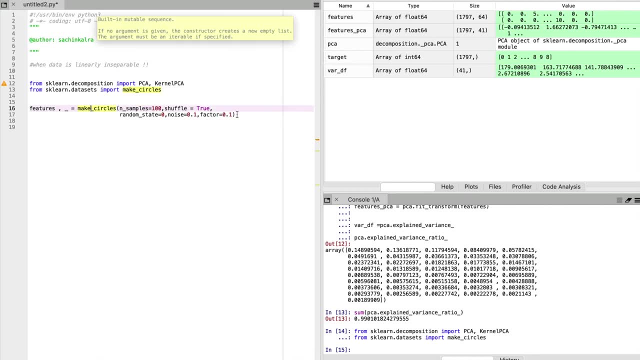 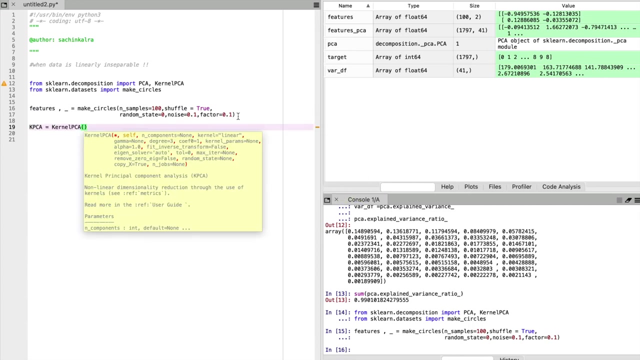 and you know you can read about how. what is a, what is this noise, what is this factor and what is this? make sure the data set. all right, I'll just run it. you've got the features with 100 rows and two columns, all right. as a next step, I'll call the kernel PCA and I'll add the kernel SRBF. see. 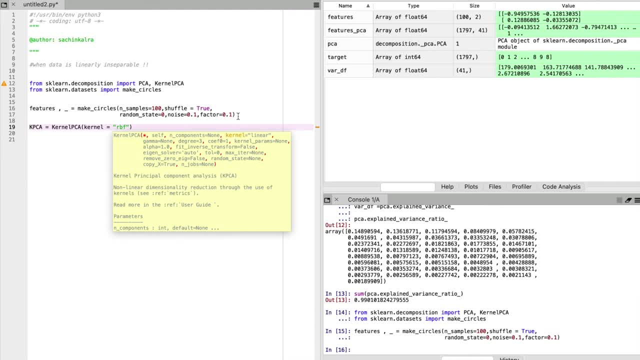 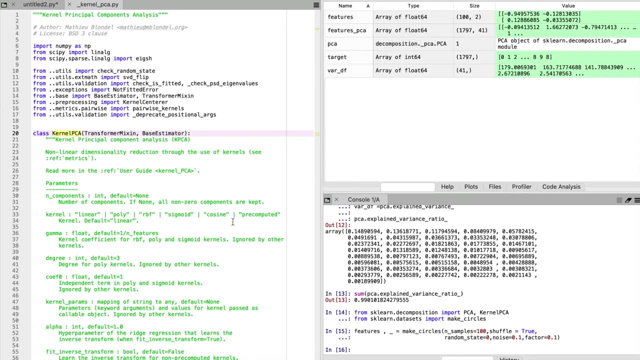 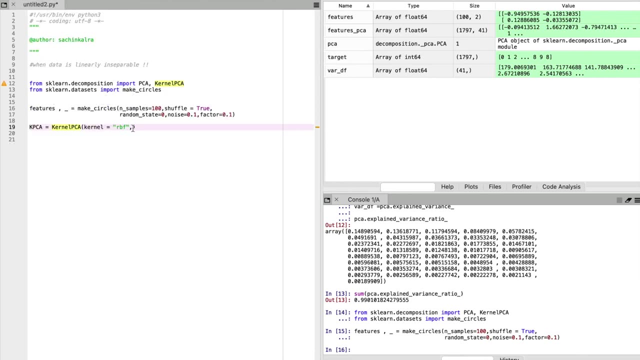 in SVM video. I have, you know, introduced it. what? what is kernel? so downside of kernel PCA is we don't have option to set, you know, percentage variance to to be retained. instead, we have other set you know number of hyper parameters in kernel PCA which which, you know, they come with own set of values, like gamma. 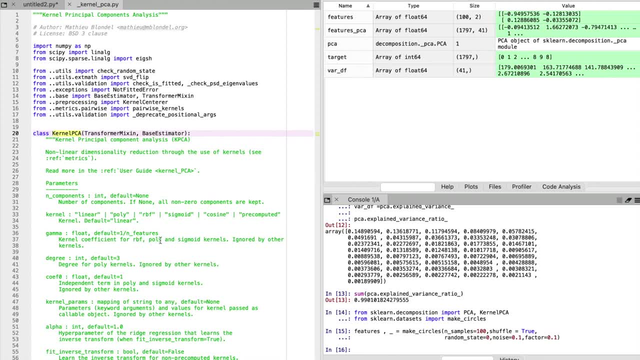 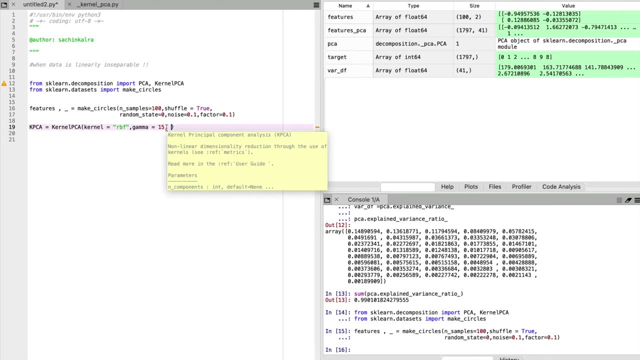 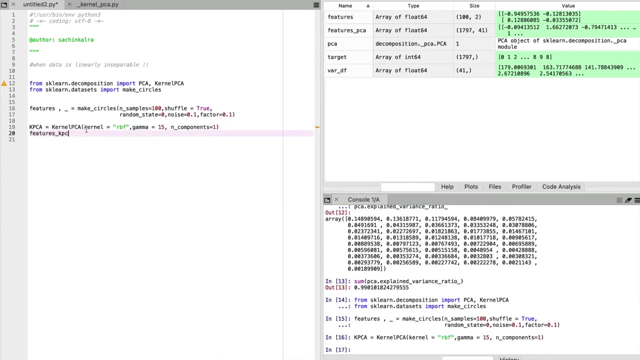 radial basis, etc. so that's how it goes on and that is, you know, just one downside. but through trial and error and grid search you know we can find the best possible value use. so for now I'll just add: I want one component out of it and let's see, we'll just, you know fit. 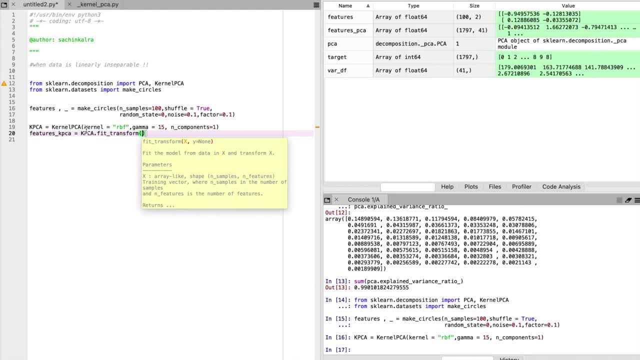 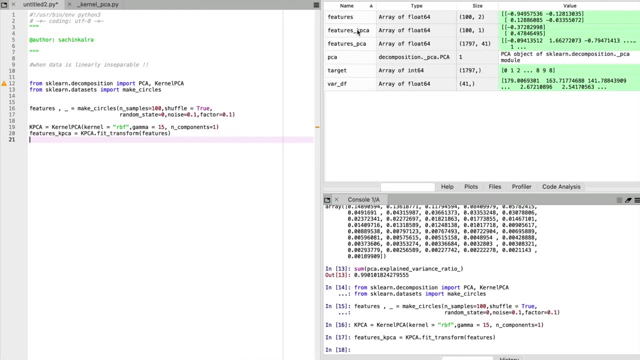 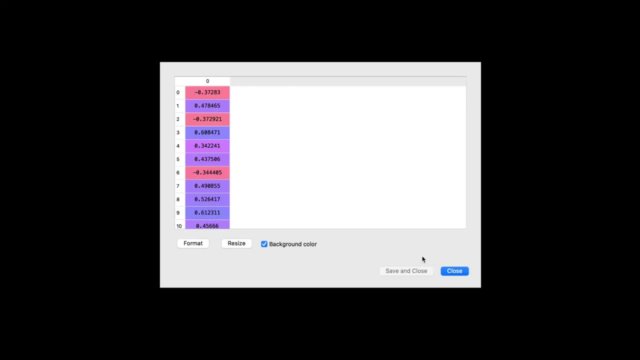 transforms it's. it's also an unsupervised technique. we'll just pass on the features through it. all right. now let's have a look. all right, we've got the features reduced to two now earlier we had- uh what? just a second, I think open the wrong window. 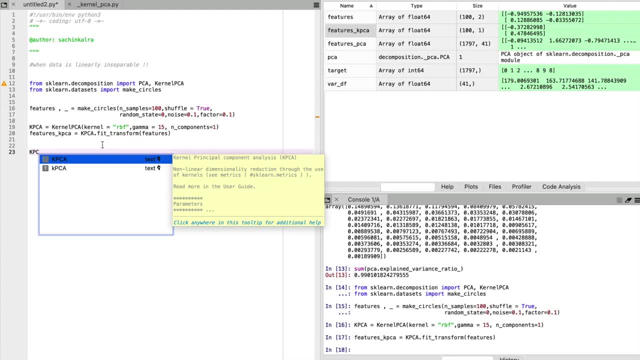 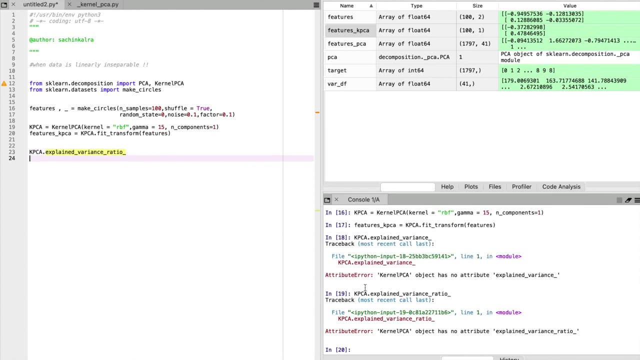 yeah, okay, our features got reduced from two to one. let me check the explain variance ratio here as well. and yeah, it doesn't have. okay, so it doesn't have the uh explained variance ratio. no worries, you can, you know, check it on the psychedelic documentation as well. what? what other attributes? 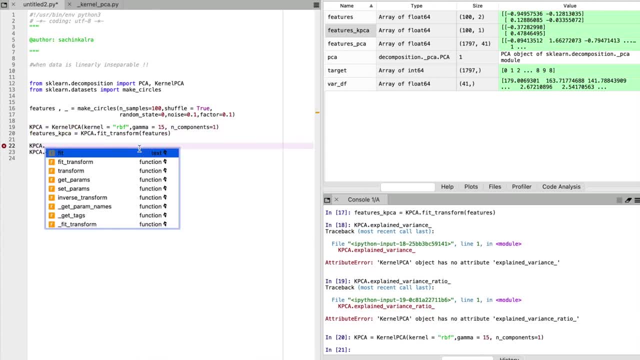 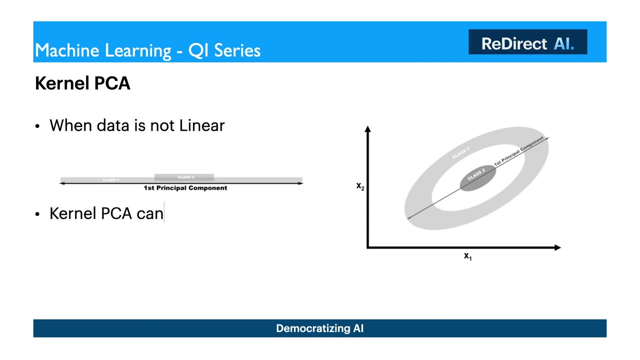 it has and even try. so yeah, this is how we did kpca and the kpc value. let's move on to the another technique called LDA. all right, so we saw how we implement PCA and kernel PCA, and let's move ahead with the next technique called. 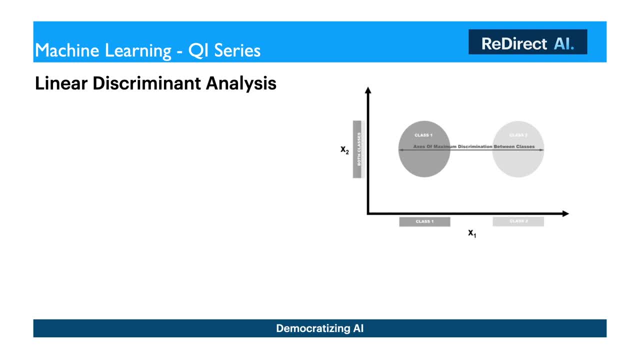 LDA. so linear discriminant analysis. it is a technique of reducing features by maximizing class separability problem. okay, so we'll try to separate out the class, the difference between two classes, and also that you know you want to reduce the features to be used by a classifier. so 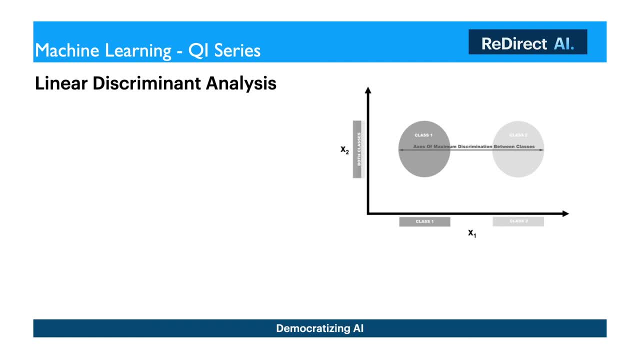 when you, when we have a classifier algorithm at hand- maybe you- we have a categorical, you know target variable, we go with the linear discriminant analysis and we try to maximize class separability. so LDA is a you know classification that is also a popular technique for dimensionality reduction. 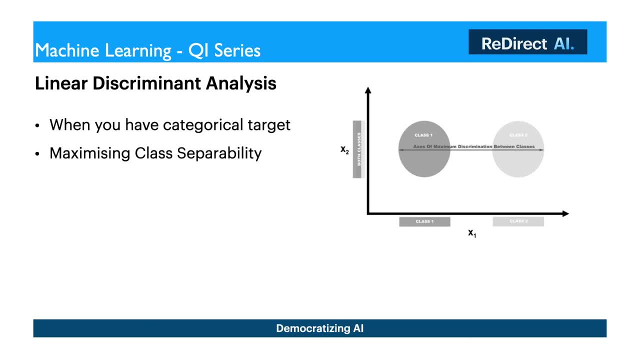 LDA works similarly to principal component analysis, in one case that it projects our feature, you know. it projects our- how do I say? it projects our feature space onto a lower dimensional space. and in see, in PCA we are only interested in the component axis that maximize the variance in the 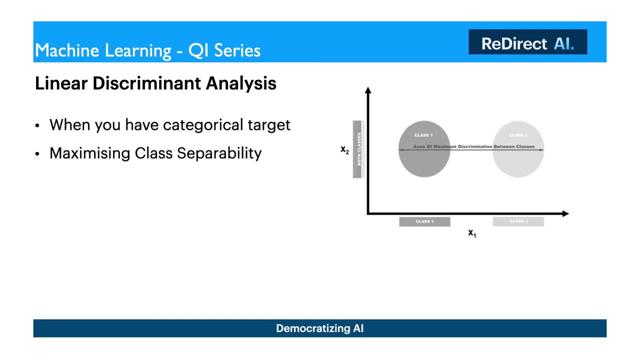 data, as we saw. but in LDA we have the additional goal of maximizing the difference between two classes. now, in this example that you see that we have class 1 and class 2, we have. you know, on x-axis we x1 dimension, we have class 1 and class 2, and in x2 we have 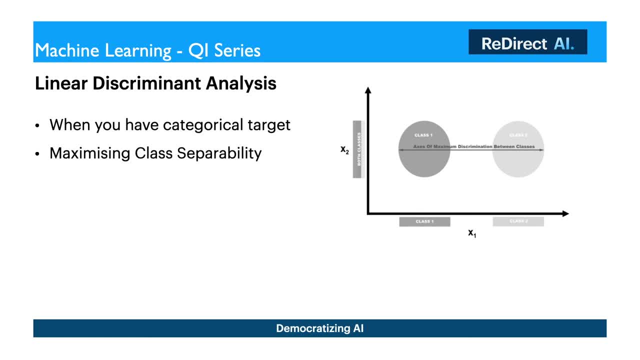 both the classes together. now in this example, let's say we have two target classes and we have two features. now if you project the data onto the y-axis, on the x2 axis the two classes are not easily separable- right, because they overlap. but while if we project the data onto the x-axis, we are left with a feature. 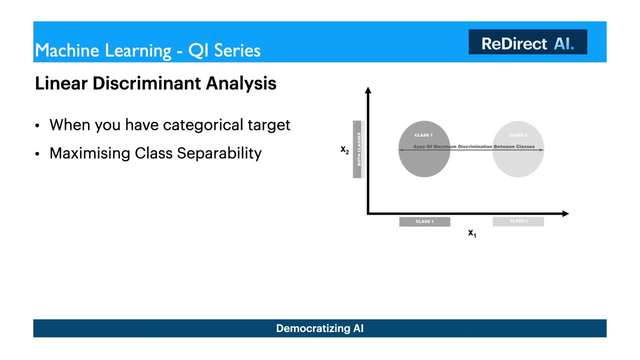 vector? definitely, they are easily separable. thus we reduce our dimensionality by one and that still preserves class separability. now, in real world, of course, the relationship between the classes will be more complex, as usual, and in dimensionality will be higher, but the concept remains the same. 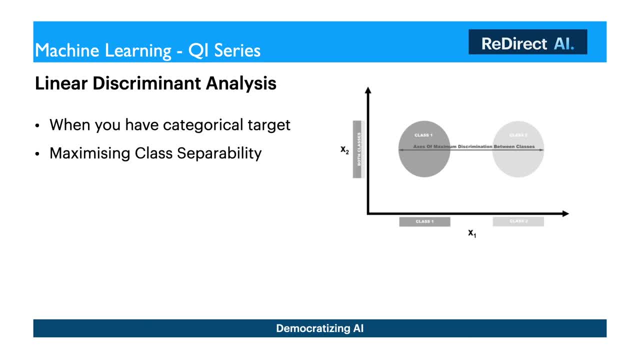 okay, so let's implement this as well and see how it goes. you know we have a. well, we can use the LDA for classification as well. I'll explain that in a separate tutorial that you know how we can use LDA classifier for a classification problem, let's implement it and see how it goes. in scikit-learn, LDA is. 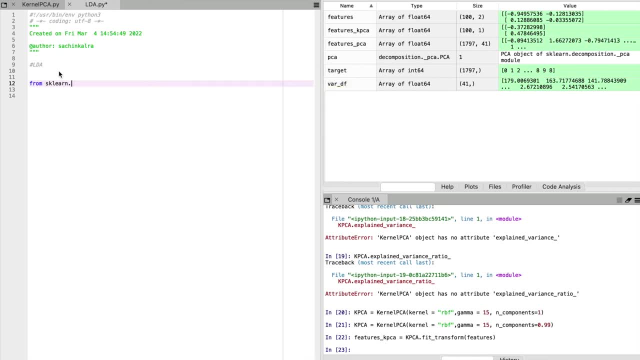 implemented using linear discriminant analysis, which includes some parameters, like n components, which indicates the number of features we want, and we have the attributes, like a explained variance ratio, which tells us the experience or variance explained by each output. So let me just call on the important libraries once again. 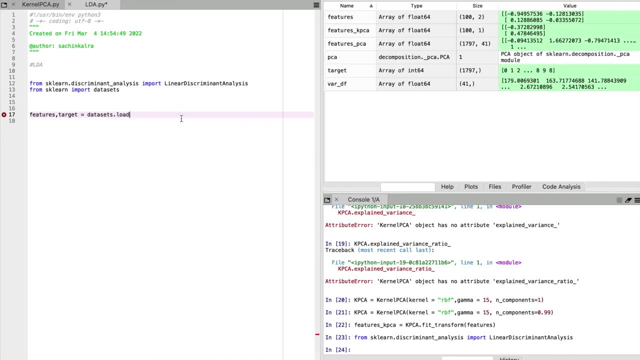 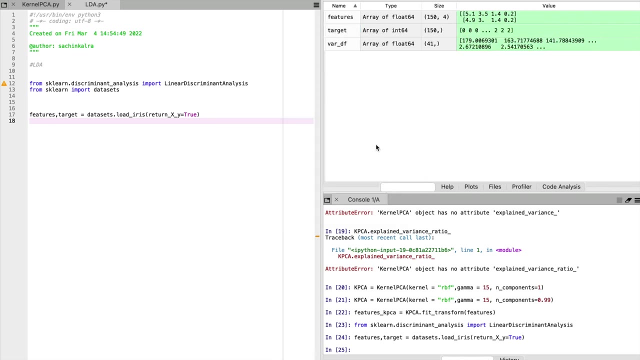 and we'll unpack features and target from the data sets, So we'll use the RSA. since LDA is used when data is going to be ingested by a classification algorithm, All right, All right, and just remove some of the redundant values. 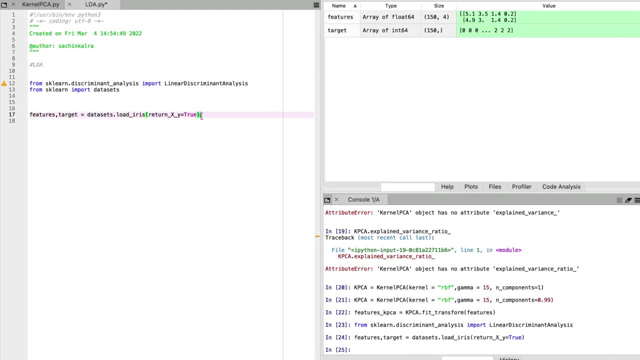 We don't want that. we don't want that. Okay, we are good, neat, All right. so I'll just call LDA and we'll just see what components it has. All right, looks very much similar- The end components. how many components do we need? 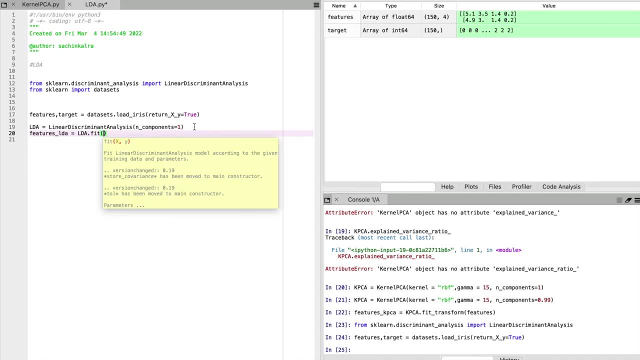 All right, we'll just fit it. So right now, while fitting it, we'll pass on the features as well as target, and then we'll transform the features. So it's a supervised technique where we learn the target classes as well. 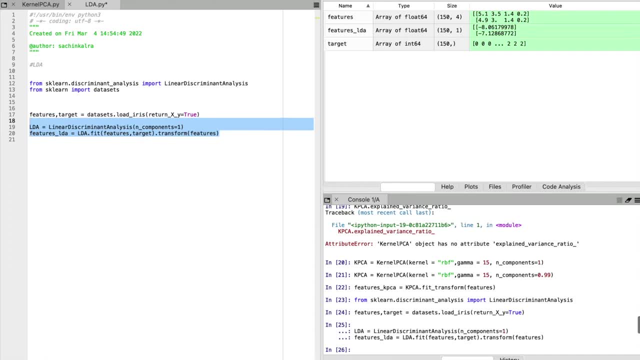 So, while fitting, we'll pass both X and Y, and to transform, to transform X, we will pass both features and target. All right, again some confusion: positive, negative, real numbers. but don't worry about it, We'll run one more, just a second. 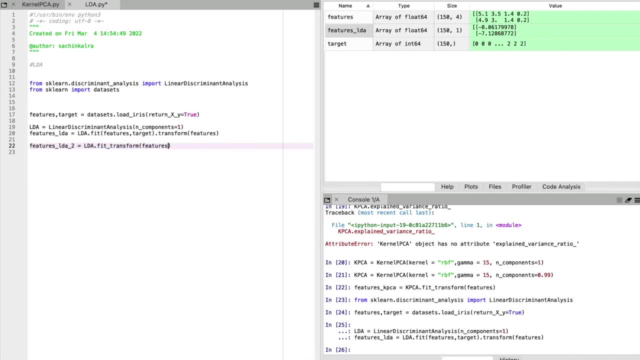 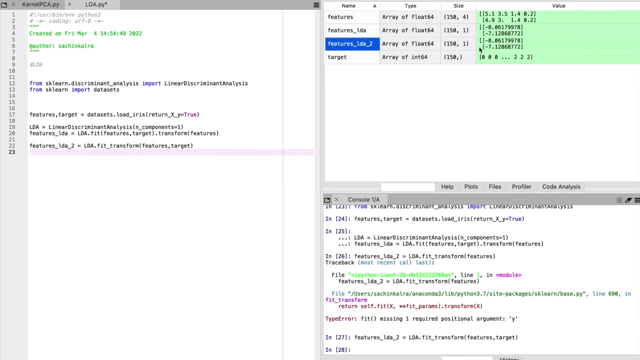 I want to show you something. Whether you know, do you have to fit and transform? so yeah, I would say that. okay, I'm missing one argument. You see, it's pretty much the same, So you can just directly use the fit and transform. 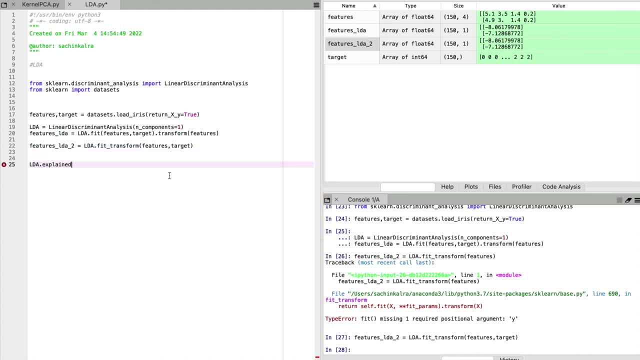 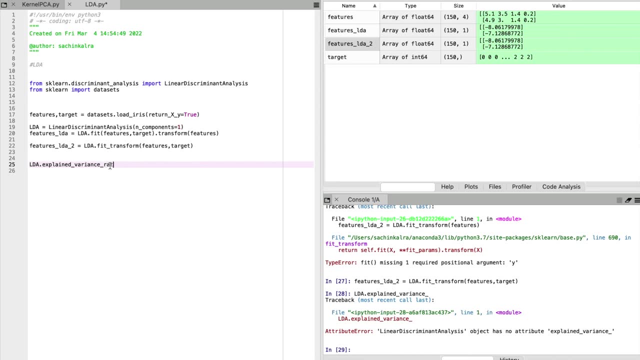 Yeah, that pretty much solves the doubt as well. All right, let's see if it has explained variance. Oh, okay, it doesn't have the explained variance. all right, I was under the impression that it has explained variance. Should have explained variance as well. 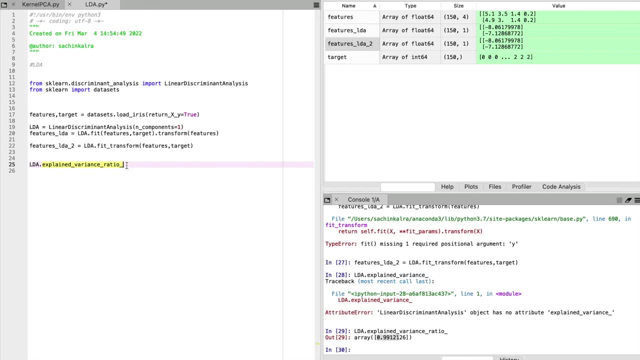 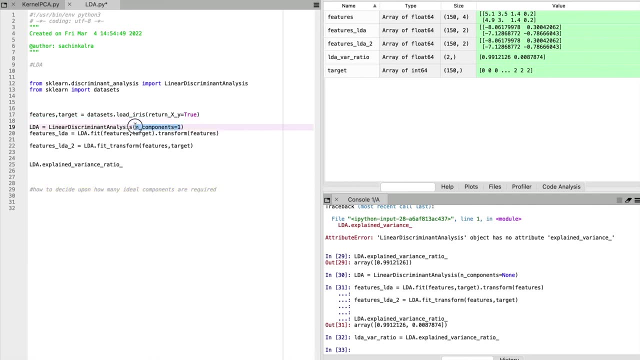 if it's able to explain the ratio, Okay, no worries. no worries, I'm just checking the implementation: How to decide upon how many idle components are required. So that is something you know. we discussed that. we will prepare a code and we can run LDA. 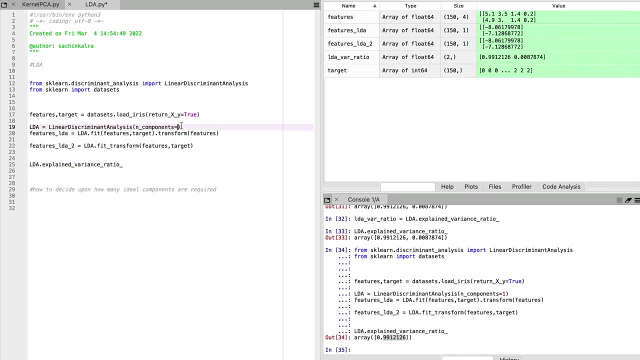 with any components you know, set to a none initially, to return the ratio of variance explained by every component feature, and then we'll, you know, calculate how many you know. just it gets too difficult, you know, while you know. 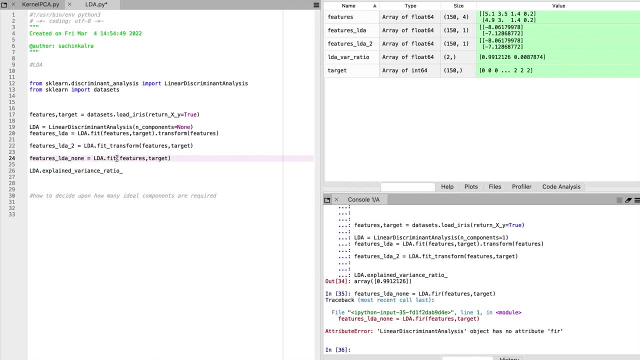 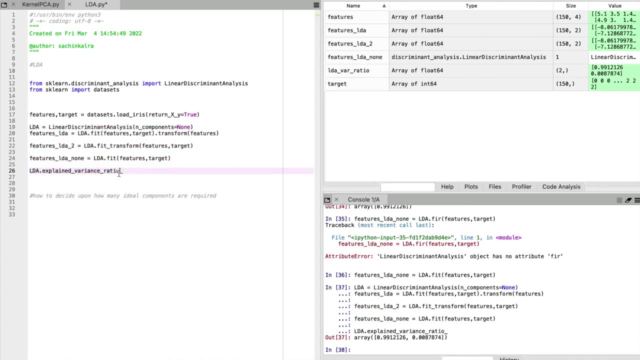 arranging and writing the code as well. Hold on, You'll just see in a moment what I'm trying to explain. So we're making the function stop the LDA once we have reached certain variance. all right, Okay, when you set the components to none. 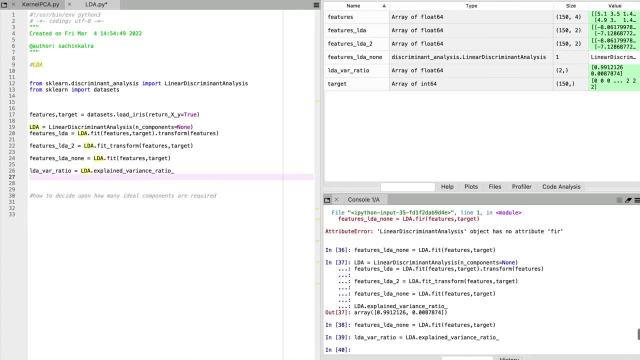 you see it has taken the automatically how many components that would be required. that is two, All right, so for two components we've got the ratio as well. you can see on the console like nine to nine, nine, zero to zero, eight percent. 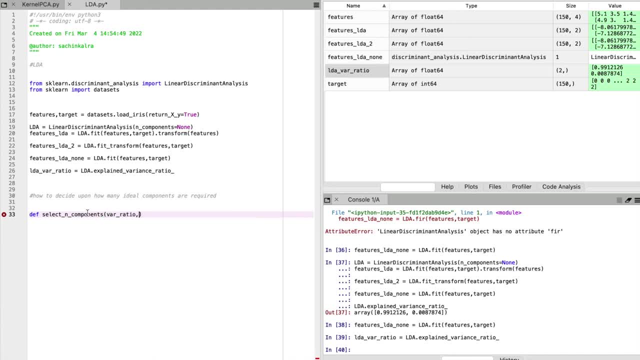 All right, now let me create a function: select in components. we'll pass in a ratio. What is our goal? variance? It should be a float, but it can take values in as well, All right, and then we'll set initial variance explained. 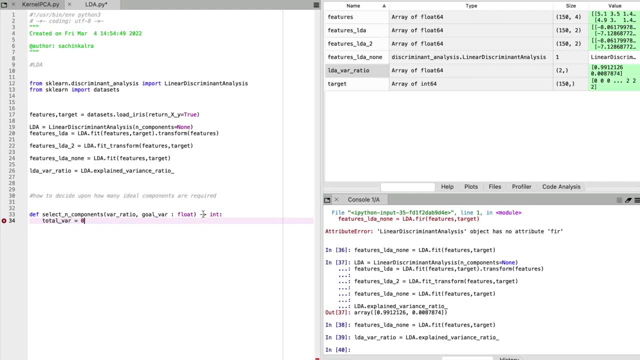 so far as total variance to zero, and then we will set number of components initially to zero. Now for explain variance in variance ratio: total variance- new total variance would be sum of the explain variance added with the total variance. So we'll just add plus equal to and yeah. 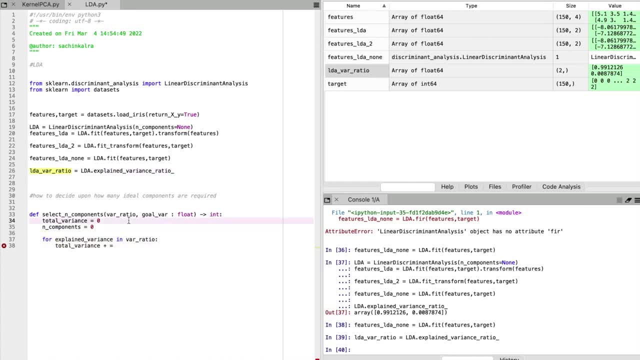 Now, once we proceed, you know we have to increase the number of components by one. I'm going a bit slow here because it's really it's a really important function. Now what happens if we reach our goal right? 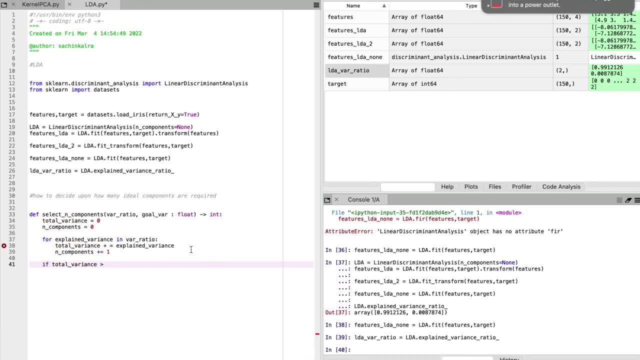 If total variance is more than or equal to our goal variance. what we'll do is we'll just, you know, I think we're good to go there, and we'll just you know, break our loop and we can print goal variance reached. 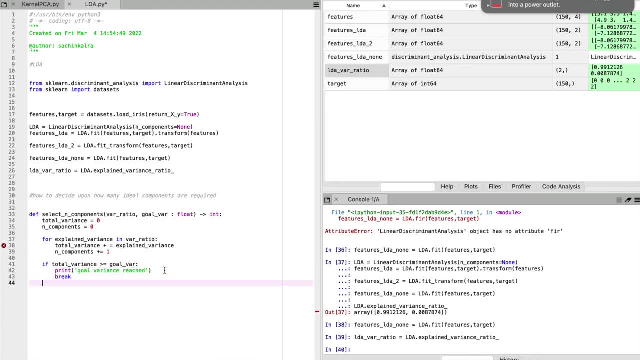 and we'll just hit break, All right, and we'll just return and components: Okay, it's going somewhere. I don't get it. What's wrong here? What's this? We click outside loop. no, it's inside the loop. 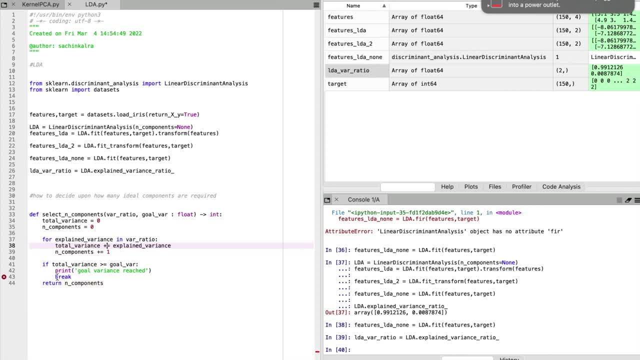 What's wrong. You know, sometimes these issues pop up during runtime as well and I'm sorry, I'm not able to remove it from our tutorial. what happens? Just bear with me for a moment, please. So these are. you know, these are like runtime errors. 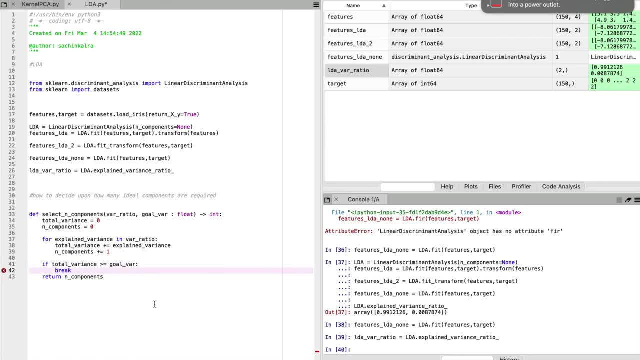 that you'll face as well. so, yeah, I think it's a good learning as well. Mm-hmm, You know, I'll just put it back. Oh okay, oh, sorry, so if is out of loop, actually, yeah. 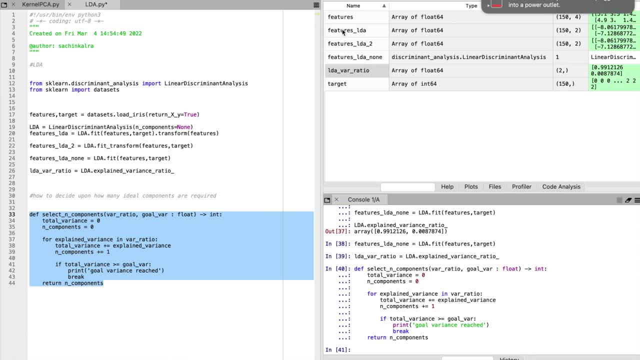 Yeah, so all right, Mm-hmm, we got a function and let's run it. Okay, I'll just call it selecting components. I'll pass in the value issue and threshold is 0.95.. I think it should stop after one, oh yeah. 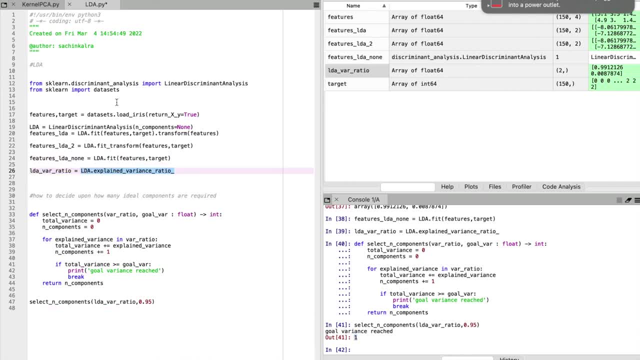 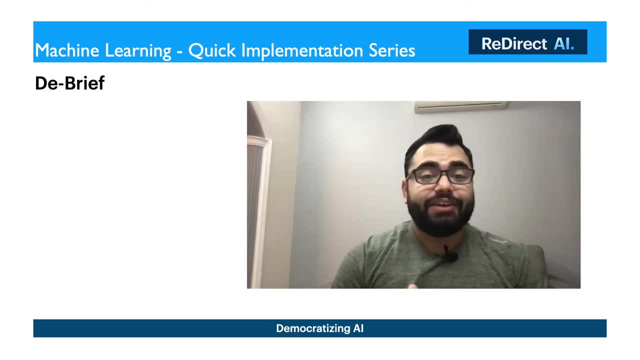 it stopped after one because we had two components only. Yeah, I think we need two components. So, yeah, this is how you know we apply LDA. All right, everyone, thank you. So today we discussed some of the very important techniques. 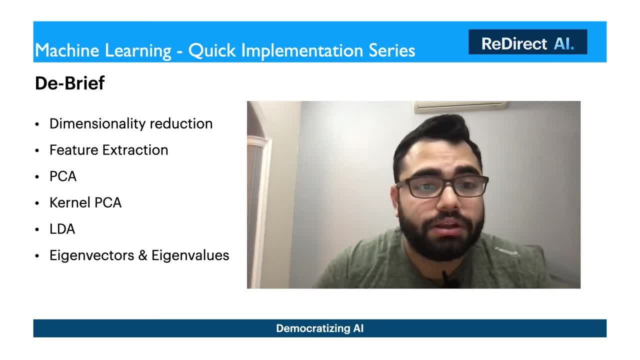 like dimensionality reduction by feature extraction, in which we saw PCA kernel, PCA LDA and what are eigenvectors and eigenvalues Now discussing about? why not? I'll just try to put in. try to put in. put it in a very simple manner as I can. this is my experience. 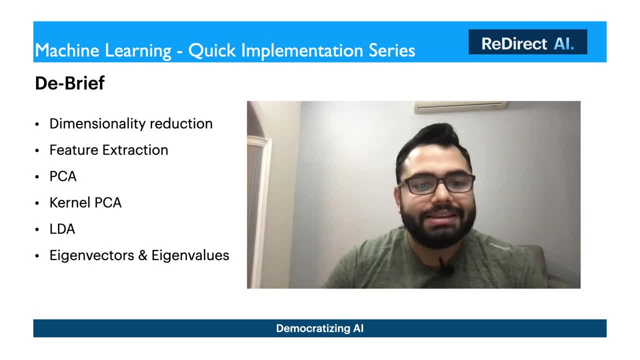 see. one key criticism of PCA is that the transformation is fairly complex and as results are therefore hard to interpret. you know, as we saw in the code as well, the principal components and the projected vectors are real valued and may be the real value, so they could be positive or negative, as we saw now. PCA: 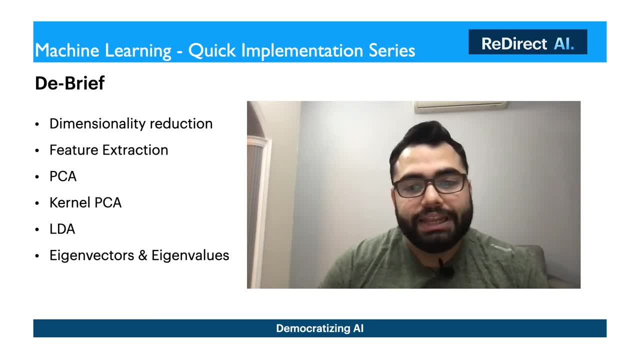 sorry, the principal components are essentially linear combinations of rows which have been centered and the projection values are also linear combination of the columns up. now, in a stock returns application, for instance, each factor is a linear combination of time slices of stock returns, definitely. now what does that mean? I mean you have some negative values, we have some. 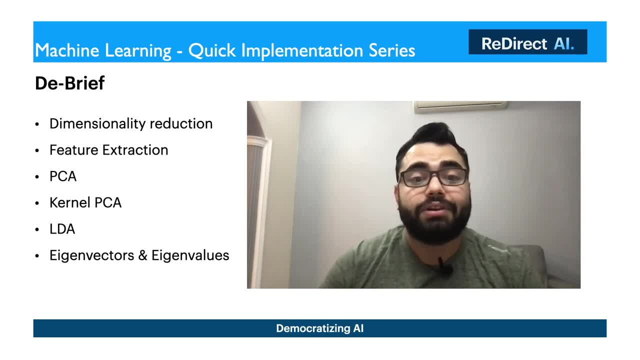 positive values and it's really hard to express- I even understandable reasons, what you learn factors. therefore, it is hard for analysts to trust the results. now, if you can't explain you know why you should be putting billions of others people money into into particular stocks? you probably won't. you know choose. you probably won't choose to, you know use. 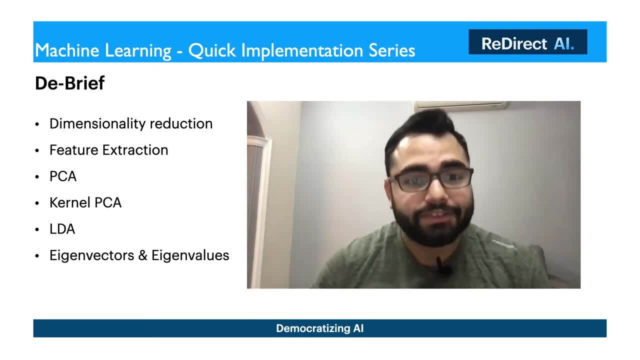 that model make sense to me. I hope it makes sense to you as well. I'm able to explain why not. we say, but yeah, it's a key criticism actually, but idly, we end up, you know, building financial index using PCA. lastly, it is not you know best. 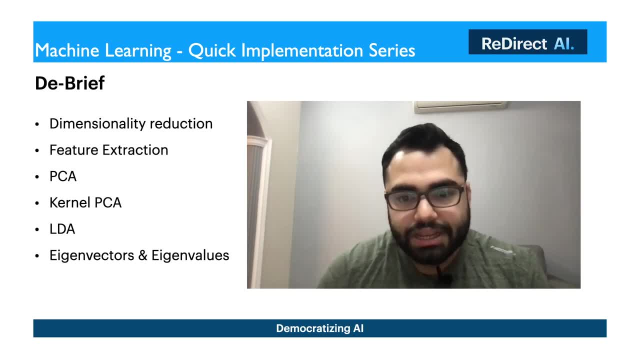 not to apply PCA to rock row counts. like you know. if you have like word counts or you have natural language processing, you have, you know, sparse matrix like that, but that doesn't mean that you should not apply it. it's a very helpful feature. I have implemented in many of my projects and you know it really helps out to.